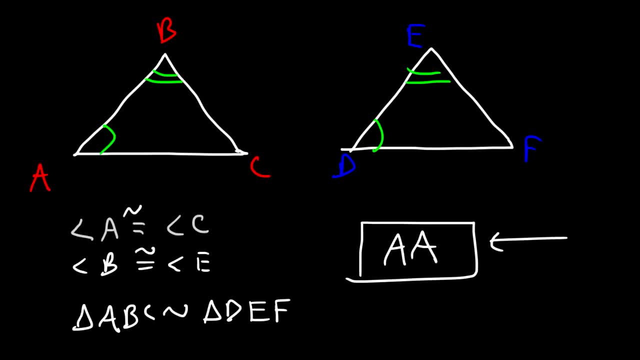 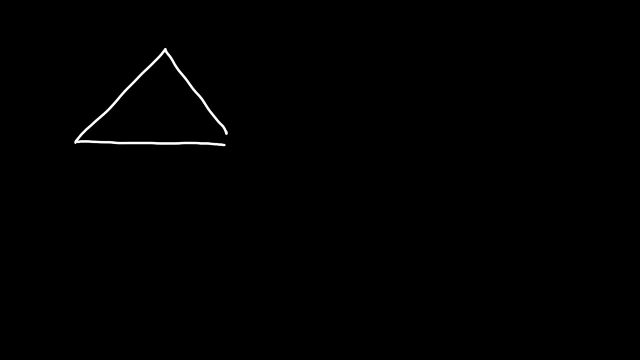 congruent. So this is the minimum work needed to show that these two triangles are congruent. Now, another method that we could use to prove that the two triangles are similar is by calculating the ratio of the corresponding sides. So if we can show that, 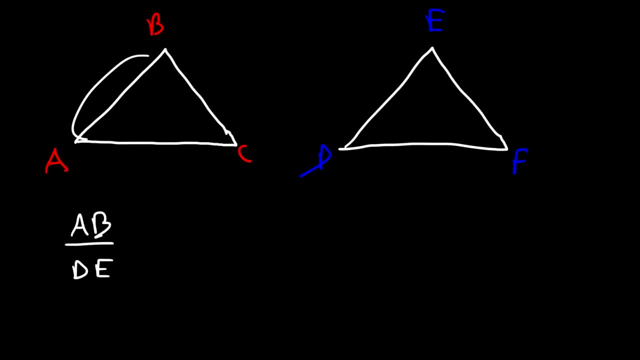 The ratio of AB and DE. these two corresponding sides have the same ratio as BC over EF, that's these two corresponding sides, and if that's equal to AC over DF, then this is enough to say that the triangle ABC is similar to triangle DEF. 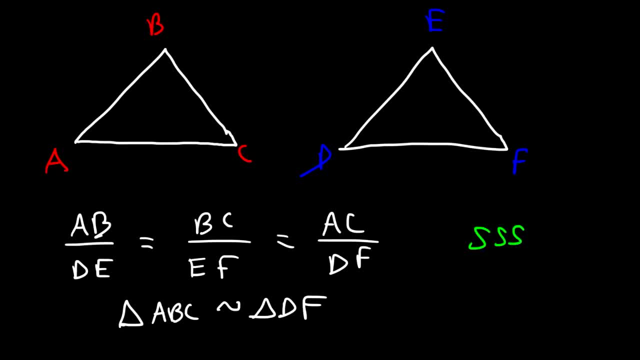 And we could use the side-side-side triangle similarity postulate. So that's another way in which you can prove if two triangles are similar. And it looks like I forgot the letter E here. Now there's one more postulate that we need to talk about. 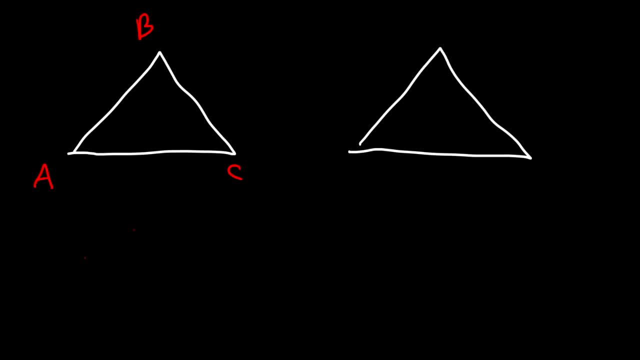 And it's the same thing. And it's the same thing And it's the side-angle-side postulate. So if we could show that angle A and angle D are congruent and if we could show that these two sides, let's say, are similar or they have the same ratio- AB and DE- as these two sides, 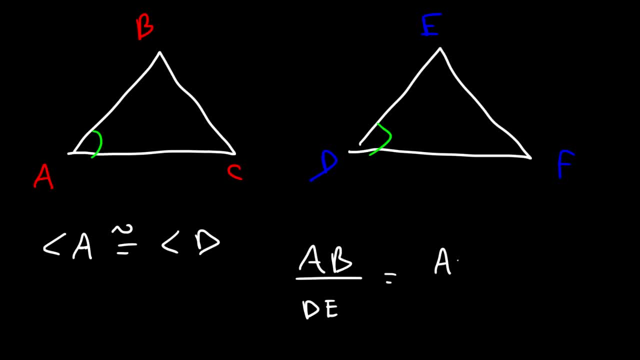 AC and DF, then, using the side-angle-side postulate, we could say that triangle ABC is similar to triangle DEF, And so that's the SAS postulate for triangle similarity. So those are the four main postulates that you can use to prove if two triangles are similar. 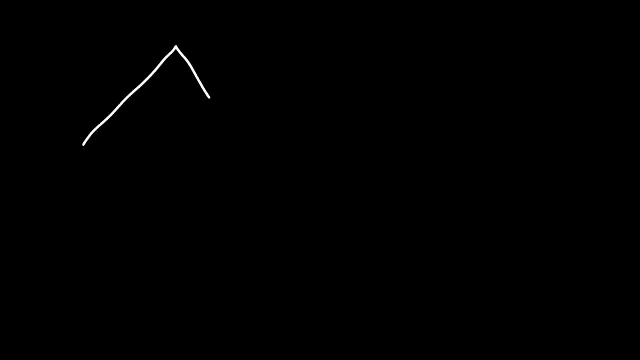 So let's work on some examples. So let's say this is triangle ABC and this is triangle DEF. So let's say AB is 12,, BC is 15, and AC is 18.. And let's say DE is 4,, EF is 5, and DF is 6.. 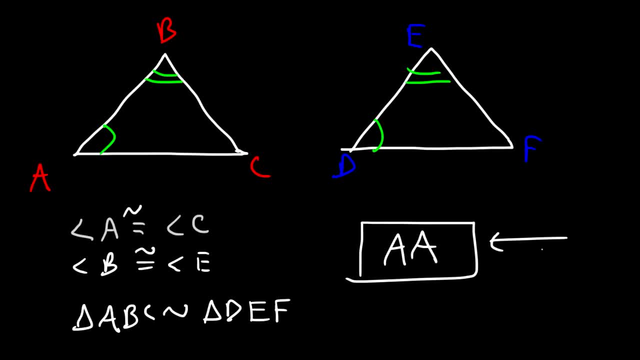 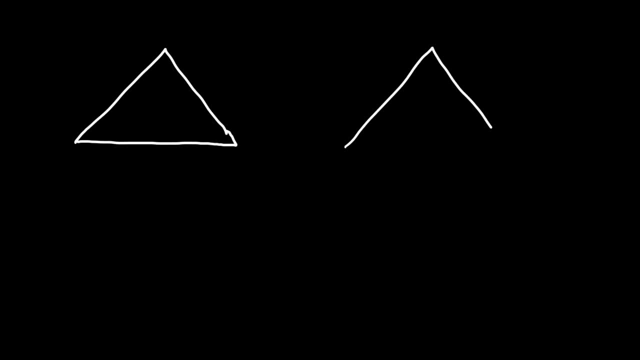 So this is the minimum work needed to show that these two triangles are congruent. Now, another method that we could use to prove that the two triangles are similar is by calculating the ratio of the corresponding sides. So if we can show that the ratio of AB and DE, these two corresponding sides have the 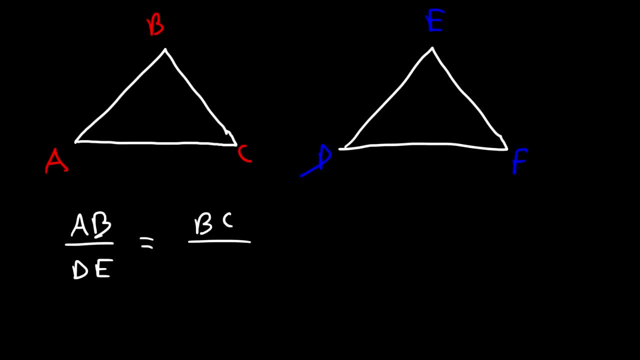 same ratio as BC over EF, that's these two corresponding sides, and if that's equal to AC over DF, Okay, Then this is enough to say that the triangle triangle ABC is similar to triangle DEF, And we could use the side-side-side triangle similarity postulate. 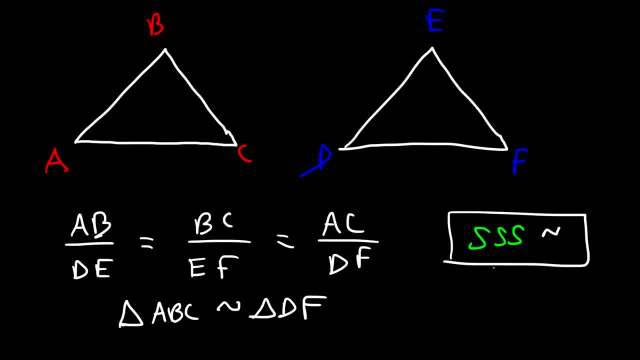 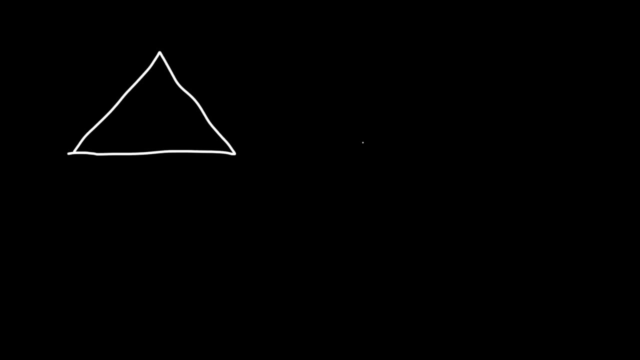 So that's another way in which you can prove if two triangles are similar. And it looks like I forgot the letter E here. Now there's one more postulate that we need to talk about. Okay, It's the side-angle-side postulate. 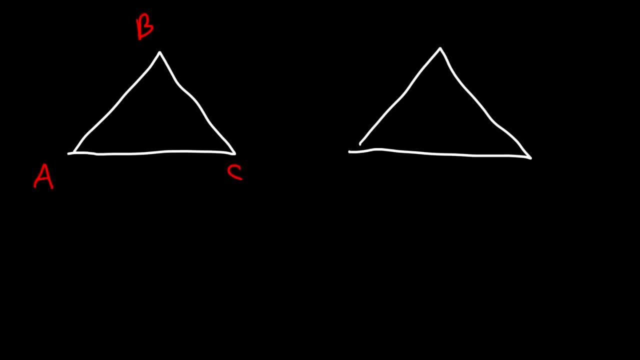 And it's the side-angle-side postulate. So if we could show that angle A and angle D are congruent And if we could show that these two sides, let's say, are similar, Okay, Or they have the same ratio- AB and DE- as these two sides, AC and DF. 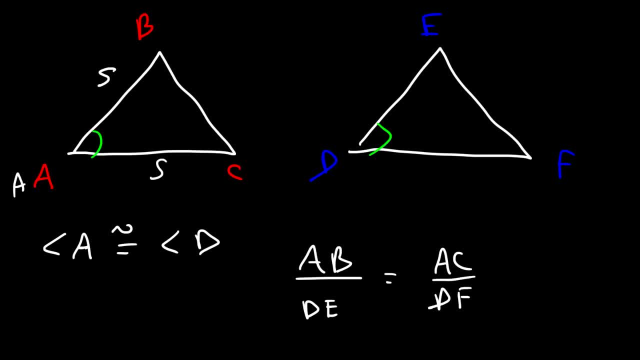 Then, using the side-angle-side postulate, we could say that triangle ABC is similar to triangle DEF, And so that's the SAS postulate. Okay, So that's the SAS postulate for triangle similarity. So those are the four main postulates that you can use to prove if two triangles are. 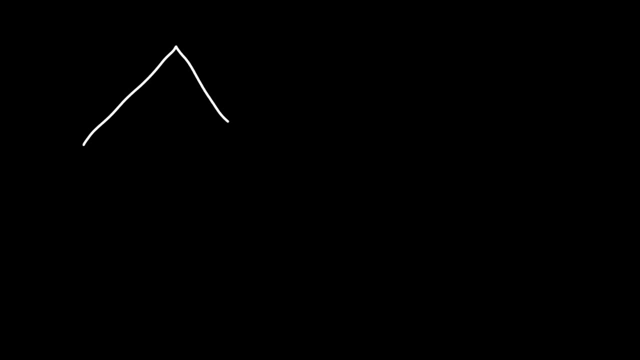 similar. So let's work on some examples. So let's say this is triangle ABC and this is triangle DEF. So let's say AB is 12,, BC is 15, and AC is 18.. Okay, Okay. So let's say these two triangles are similar. 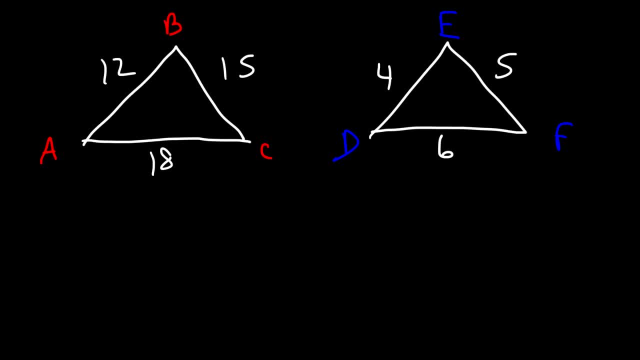 And let's say DE is 4,, EF is 5, and DF is 6.. So are these two triangles similar? And also, what postulate would you use to prove if they're similar? So first let's find the ratio between AB and DE. 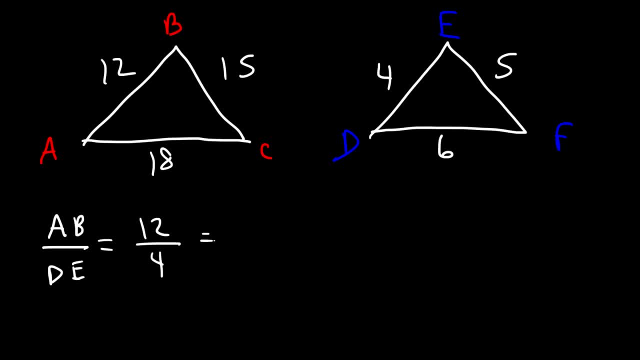 AB is 12, and the corresponding side is 4.. So the ratio between these two triangles is 3.. And then if we divide BC by EF, Okay, BC is 15,, EF is 5. If we divide those, that's 3.. 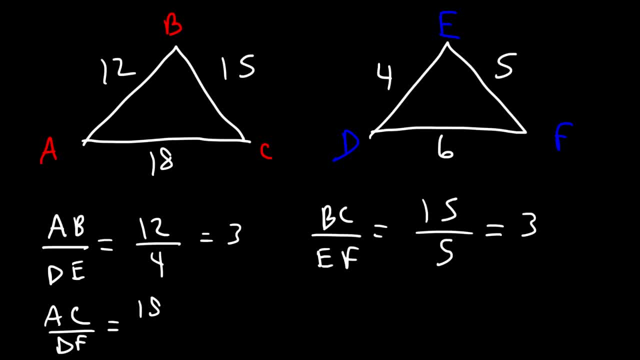 And AC divided by DF, AC is 18,, DF is 6.. If we divide those, that's 3.. So we can make the statement that AB over DE is equal to BC over EF, which is equal to AC over DF. 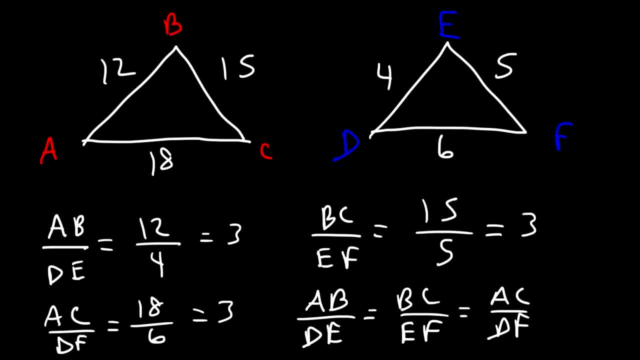 So now that we've shown that the ratio Okay of the corresponding sides of these two triangles are equal to each other, we can make the statement that triangle ABC is similar to triangle DEF, And so the postulate that we can use is the side-side-side triangle similarity postulate. 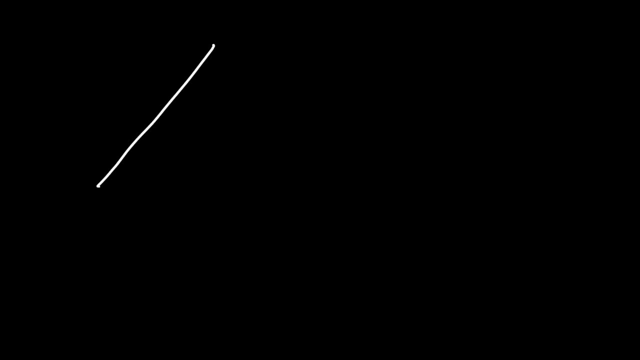 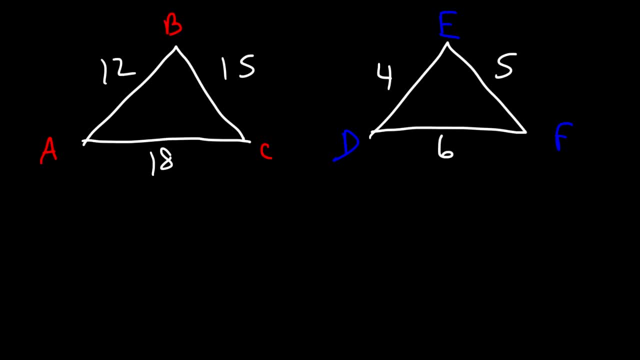 So are these two triangles similar? And also, what postulate would you use to prove if they're similar? So first let's find the ratio between AB and DE. AB is 12, and the corresponding side is 4.. So the ratio between these two triangles is 3.. 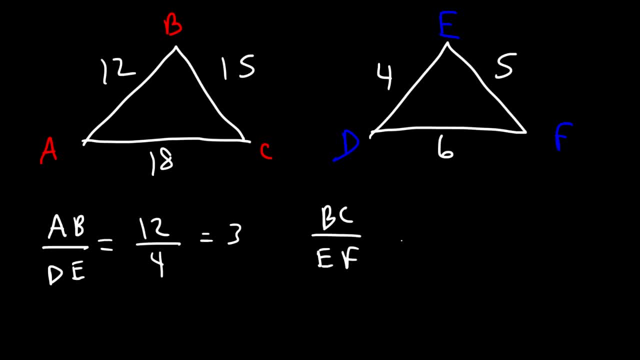 And then if we divide BC by EF, BC is 15,, EF is 5.. If we divide those, that's 3.. And AC divided by DF, AC is 18,, DF is 6.. If we divide those, that's 3.. 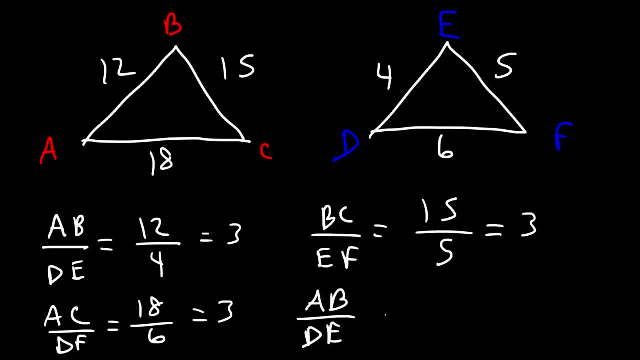 So we can make the statement that AB over DE is equal to BC over EF, which is equal to AC over DF. So now that we've shown that the ratio of the corresponding sides of these two triangles are equal to each other, we can make the statement that triangle ABC is similar. 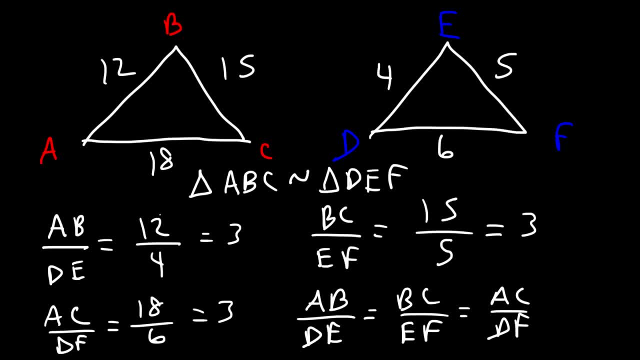 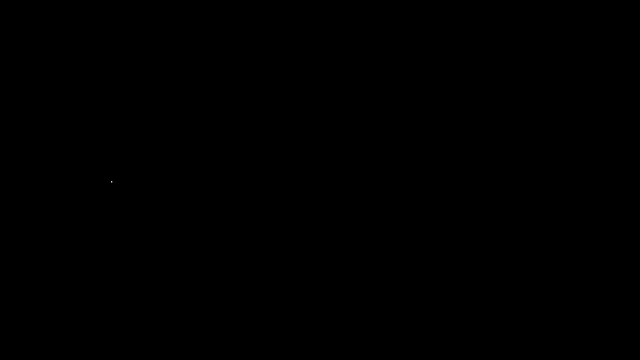 and triangle DEF is similar to triangle DEF, And so the postulate that we can use is the side-side-side triangle similarity postulate. Now let's try another example. So let's say this is angle A, B and C. Let's say we have this line: 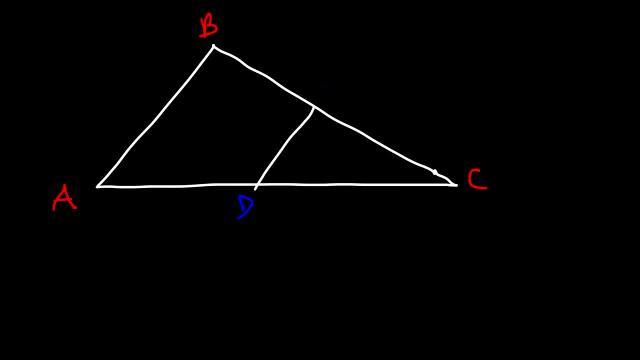 And let's say this is D and E. Let's say that DC is 7, and EC is 12.. And AD is 14, and BE is 24.. So are there two triangles that are similar And if so, what are the two triangles? 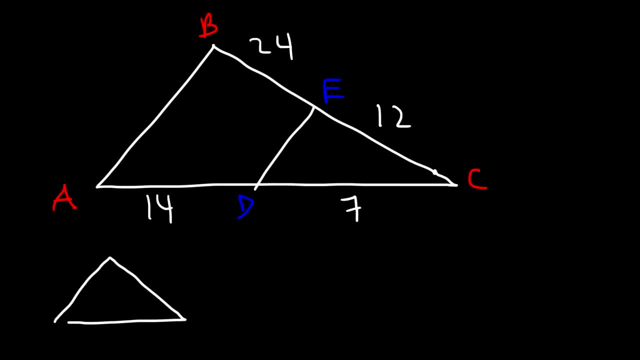 Now let's focus on the small triangle, which is DE, And also the large triangle, which is ABC. So notice that DC is 7,, EC is 12.. AC is the sum of 14 and 7,, so that's 21.. 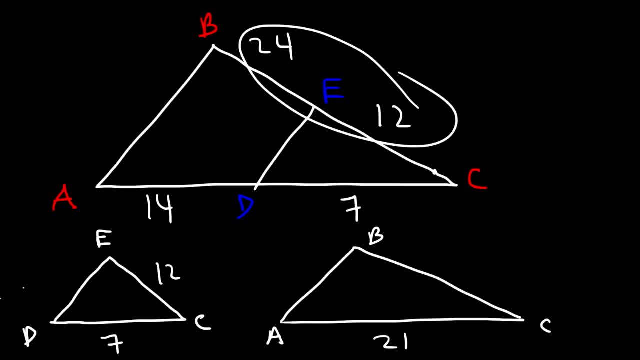 And BC is the sum of 24 and 12, which is 36.. And notice that they share a common side, That is angle C. So first we can show that angle C is congruent. AC is congruent to angle C. 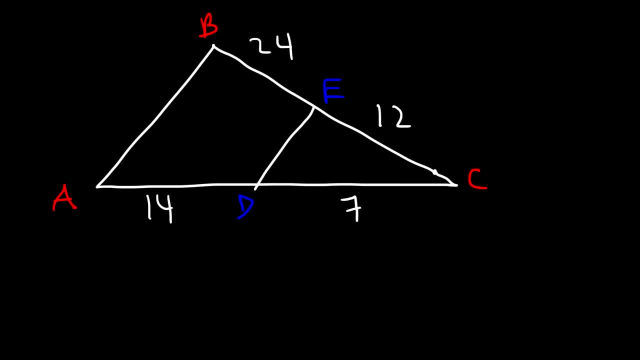 14, and BE is 24.. So are there two triangles that are similar and, if so, what are the two triangles? now let's focus on a small triangle, which is DEC, and also the large triangle, which is ABC. so notice that DC is 7, EC is 12, AC is the sum of 14 and 7, so that's 21, and BC is the sum of 24 and. 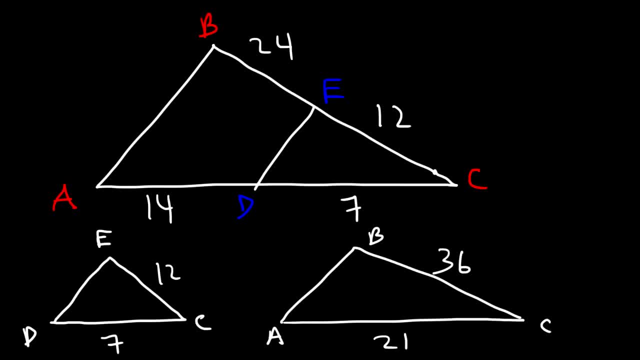 12, which is 36, and notice that they share a common side, that is, angle C. so first we can show that angle C is congruent to angle C. that's the first thing we need to do, and once we've established that, we can also see that AC. 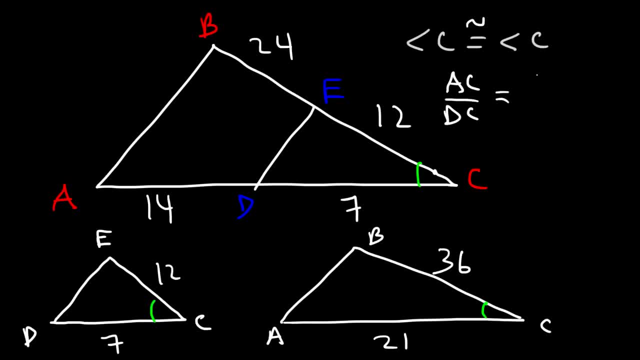 divided by DC has the same ratio: it's 21 over 7, which is 3, and so and then we could say that DEC is the same as AC, and so that's the first thing we need to do, and so, and then we could say that DEC is the same ratio: it's 21 over 7, which is 3, and so and then we could say: 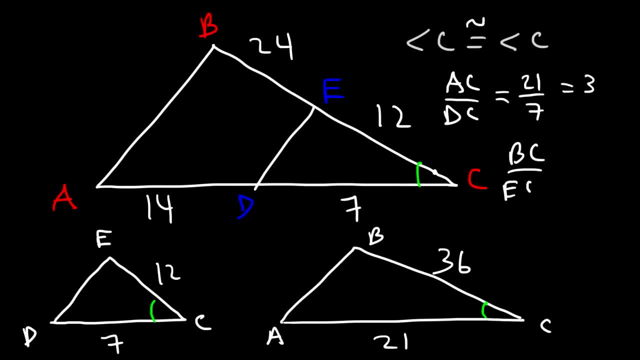 that BC over EC, that's 36 over 12, which is 3. so now we can make the statement that AC over DC is equal to BC over EC. so we've shown that the angles, angle C, is congruent and that these two sides have the same ratio as these two sides. so we can prove that the triangles are. 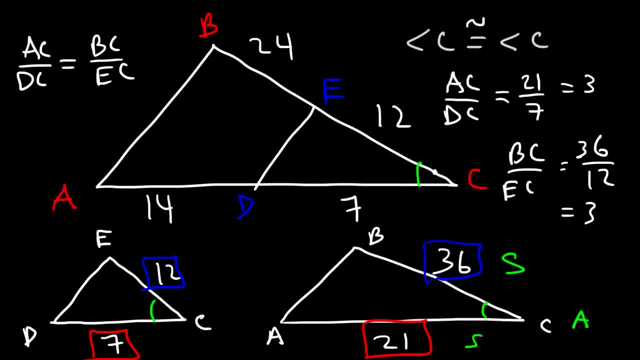 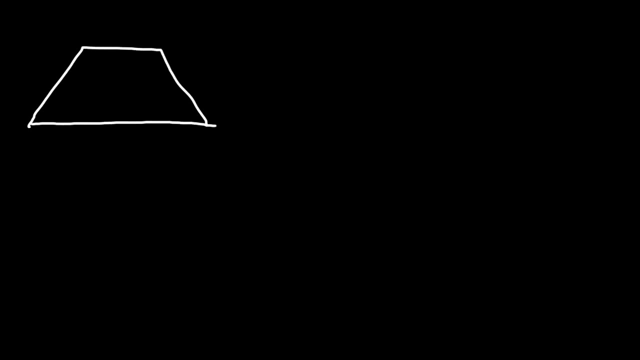 similar based on the side angle side triangle similarity postulate. so it's based on SAS and so we can make the final statement that triangle a BC is similar to triangle DEC. now let's work on triangle OBC. out a simple two-column proof using what we learn. 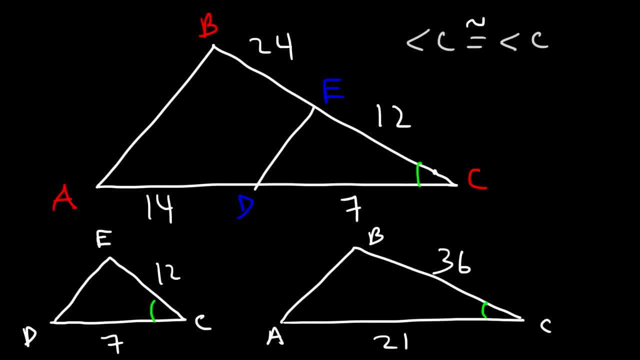 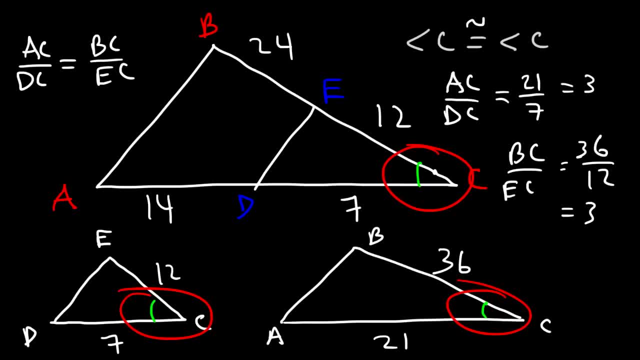 vocalize: the angle c is pretty puedan to BC over EC. So we've shown that anomaly. Now let's calculate the angles at vraag consideration. Angles, angle c is congruent and that these two sides have the same ratio as these two. 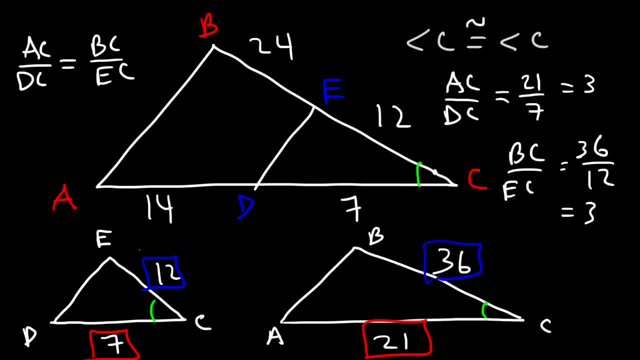 sides. This is not a very good idea, but it's a pretty awesome비 against the same as this. So we can prove that the triangles are similar based on the side angle, side outside angle similarity part. so it's based on SAS and so we can make the final statement that triangle ABC is. 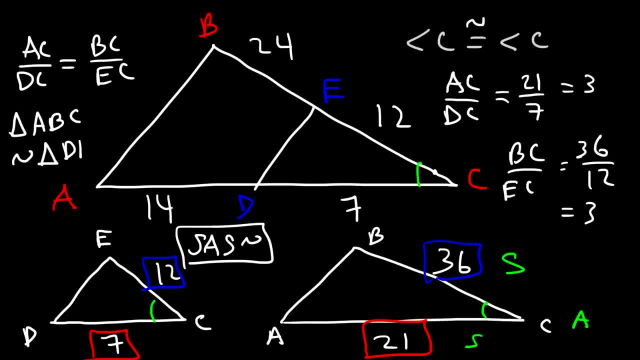 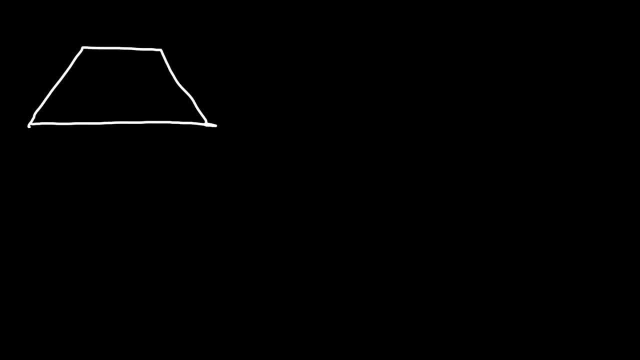 similar to triangle DEC. now let's work on a simple two-column proof using what we learn and let's say this is so in this problem. we're given this information. let's say that ABCD is an isosceles trapezoid and, with this information, go ahead and prove that triangle BEC is similar to. 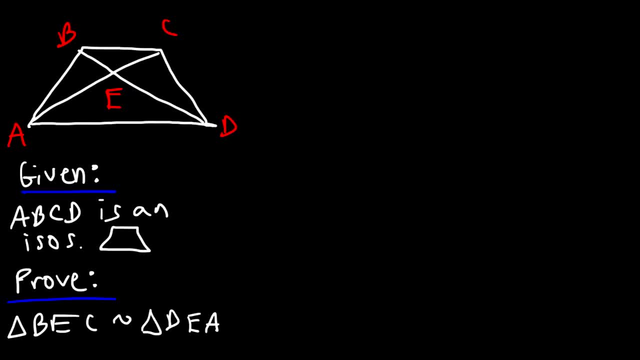 triangle DEA. so use a two-column proof to show that. so first let's rewrite our given statement. so ABCD is an isosceles trapezoid. isosceles trapezoids have legs that are congruent, and also the lower base angles are congruent as well. even the upper base angles are congruent. so 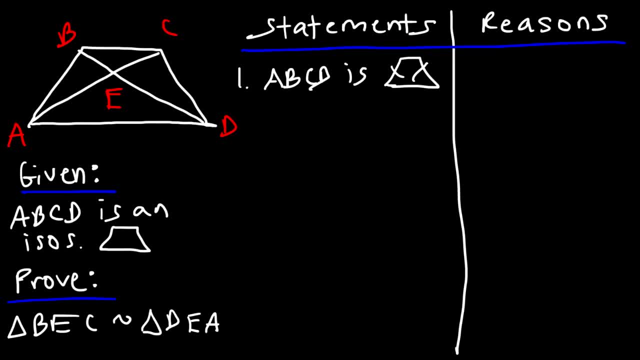 those are some basic properties of an isosceles trapezoid, and this is given to us. now let's move on to number two. what do you think we could do next to prove that these two triangles are congruent, that's BEC and DEA? for one thing, notice that the vertical angles are congruent. 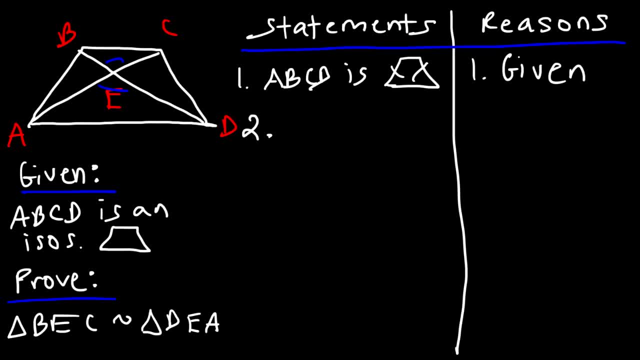 and also we could show that angle EAD is congruent to angle ECB, if we could show that these lines are parallel and the bases for any type of isosceles trapezoid are always parallel. so let's say that BC is parallel to AD, and so what we could say is that bases 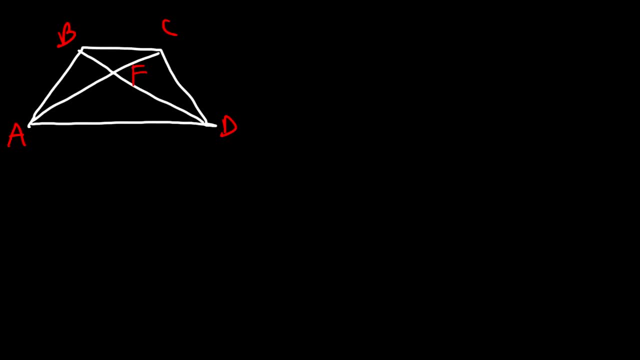 and let's say this is E. so in this problem we're given this information, let's say that ABCD is an isosceles trapezoid and with this information, and go ahead and prove that this information is an isosceles trapezoid and with this information, go ahead and prove that. 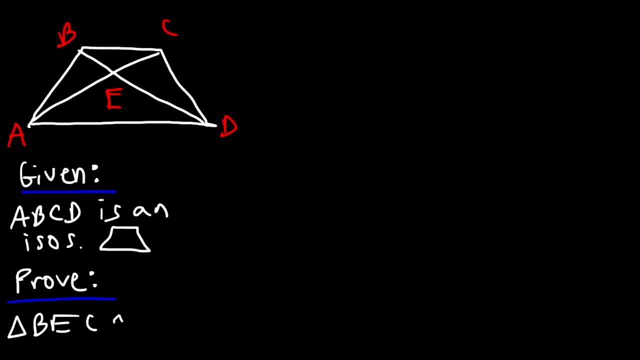 triangle BEC is similar to triangle DEA, so use a two-column proof to show that. so first let's rewrite our given statement. so ABCD is an isosceles trapezoid, is 羽繩 is an isosceles trapezoid, is dieses triangle dice. 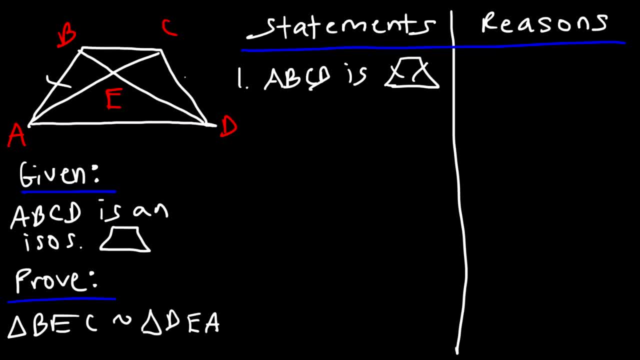 isosceles trapezoids have legs that are congruent and also the lower base angles. cc isosceles trapezoids have legs that are congruent, and also the lower base angles are congruent as well, and also the lower base angles. 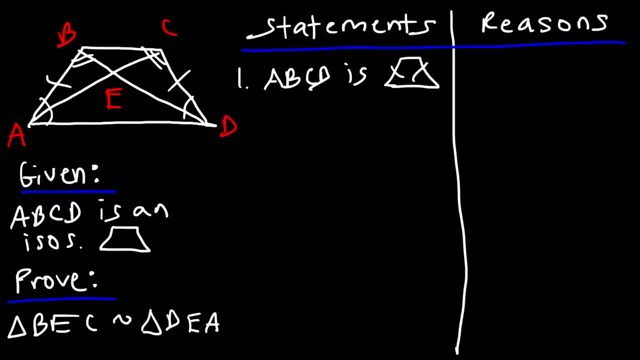 even the upper base angles are congruent. so those are some basic properties of lar isosceles. is the das musulmane of delivers? former Maya analysis, ill seen from lift el r? al. now let's move onto number two, T. well, what do you think we could do here? 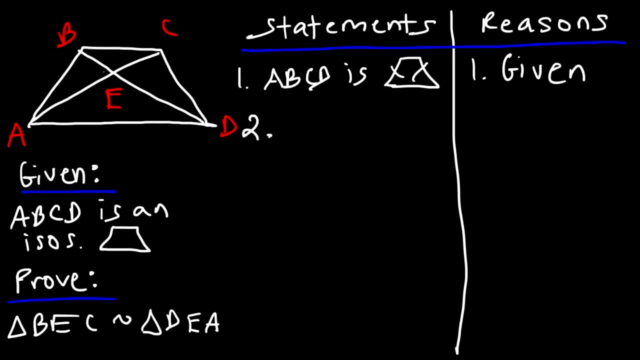 Enemy next, to prove that these two triangles are congruent. so that's BEC and DEA. for one thing, notice that the vertical angles are congruent. and also we could show that angle EAD is congruent to angle ECB if we could show that these lines are parallel. and the bases for any type of isosceles, trapezoid, are always. 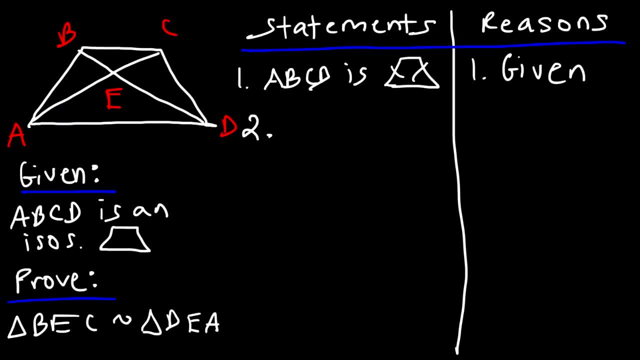 parallel. so let's say that BC is parallel to AD, and so what we could say is that bases of an isosceles trapezoid are parallel, and so let's mark that in their figure. so BC and AD are parallel. now number three we can now make: 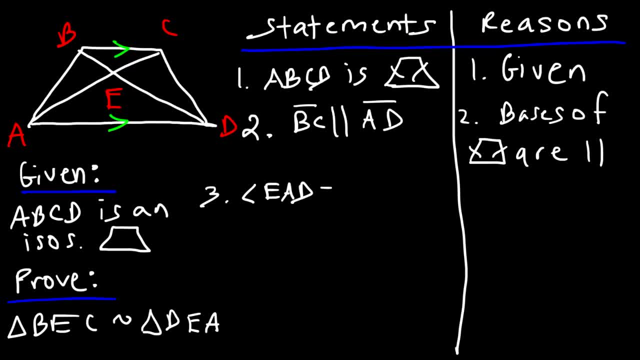 the statement that angle EAD is congruent to angle ECB. so this is angle EAD and that's congruent to angle ECB, which is here. and the reason that we could say this is that if we have parallel lines, then the alternate interior angles are congruent. here are the two parallel: 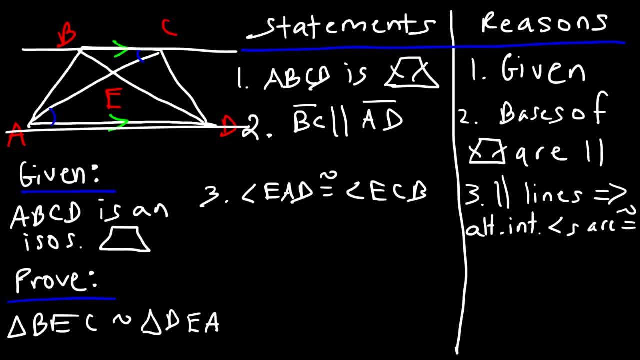 lines and these are alternate interior angles which are congruent if the lines are parallel. so now let's move on to our fourth statement, and that is that angle BEC is congruent to angle DEA. so this is BEC and this is DEA. so we know that these two, they form vertical. 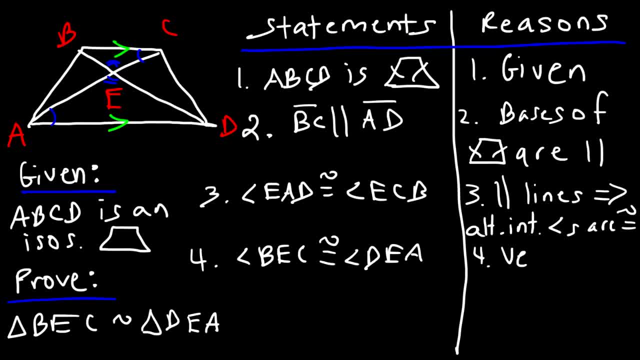 angles. and so in step four, we can say that vertical angles are congruent. so now step five, our final statement: triangle BEC is similar to triangle DEA, and- And this is based on the angle-angle postulate, because we've shown that two angles are congruent in both triangles- 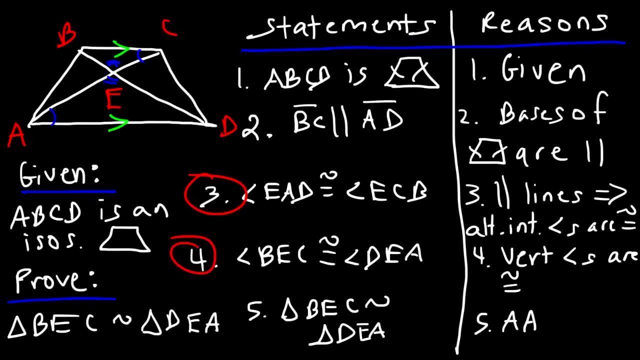 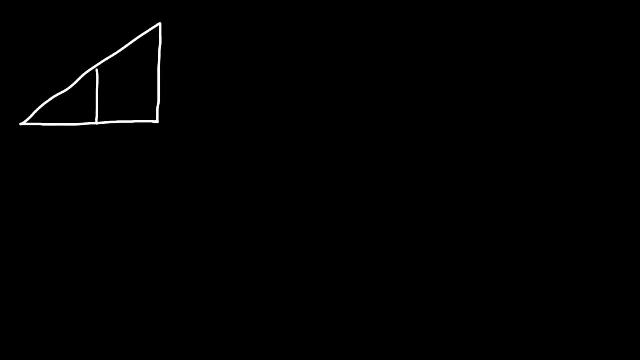 And we've shown that using statements doing four. And so that's a simple way in which you can prove that two triangles are similar using a two-column proof. Now let's work on another example. So let's say this is triangle ABC, and here we have, let's say, this is D and this is E. 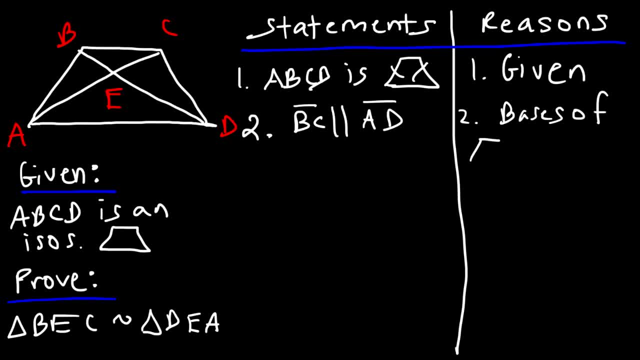 of an isosceles trapezoid are parallel, and so let's mark that in there figure. so BC and AD are parallel. now number three. we can now make the statement that angle EAD is congruent to angle ECB. so this is angle EAD and that's congruent to angle ECB, which is: 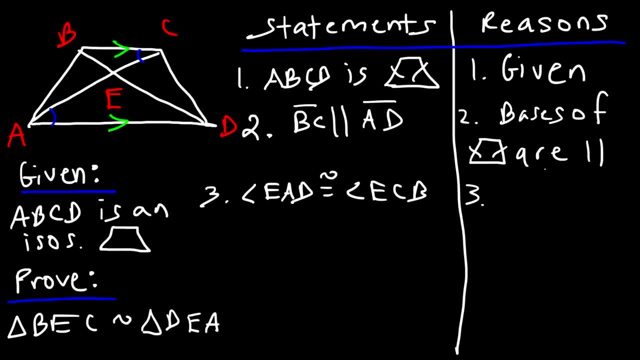 here, and the reason That we could say this is that if we have parallel lines, then the alternate interior angles are congruent. Here are the two parallel lines, and these are alternate interior angles which are congruent if the lines are parallel. So now let's move on to our fourth statement. 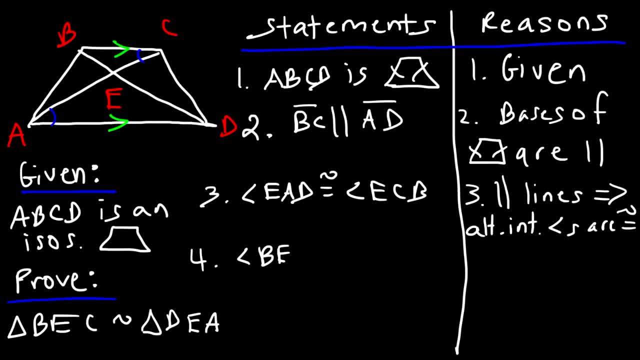 And that is that angle BEC is congruent to angle DEA. So this is BEC and this is DEA. So we know that these two they form vertical angles, And so in step four we can say that vertical angles are congruent. 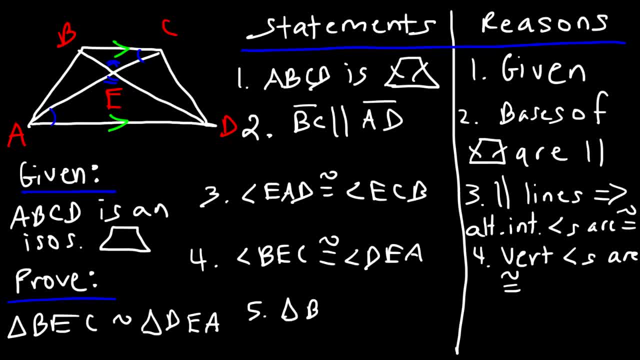 So now step five, our final statement. Triangle BEC is similar to triangle DEA, And this is based on the angle-angle postulate, because we've shown that two angles are congruent in both triangles, And we've shown that using statements doing four. 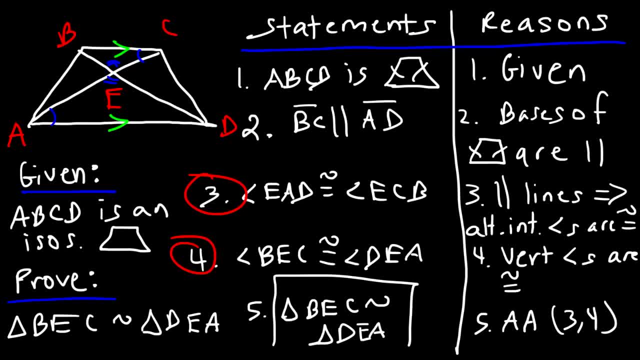 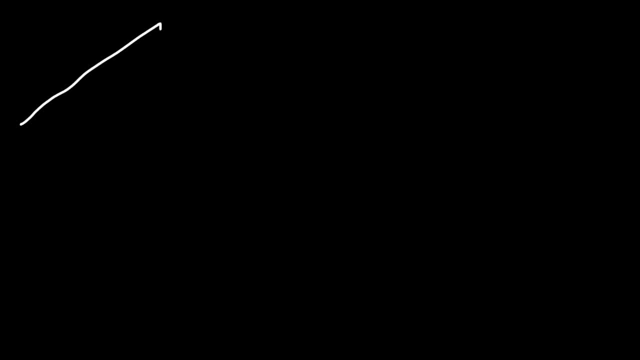 And so that's a simple way in which you can prove that two triangles are similar using a two-column proof. Now let's work on another example. So let's say this is triangle ABC. And here we have. let's say, this is D and this is E. 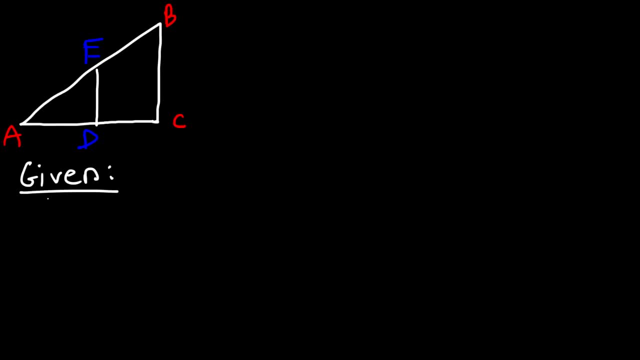 So for this problem, we're given the following information, And that is that AB divided by AE is equal to A. So for this problem, we're given the following information: So AC divided by AD. So your task is to prove that triangle AED is similar to triangle ABC. 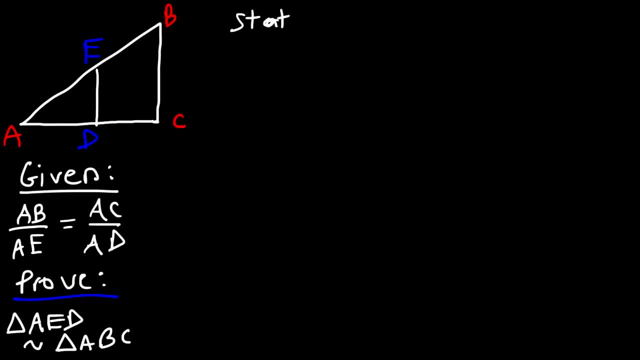 So let's use a two-column proof If you want to go ahead and try this problem. So let's start with the given, And that is: AB divided by AE is equal to AC over AD. Now let's draw the two triangles together. 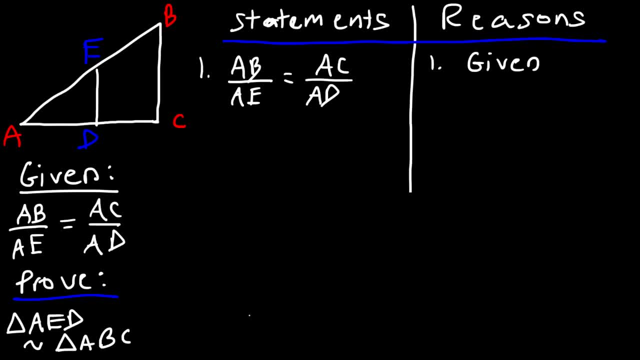 So we're trying to prove that AED is similar to ABC, So this is ABC And this is AED. Now, AB divided by AE is equal to AC divided by AD, So those two corresponding sides have the same ratio. based on this equation, 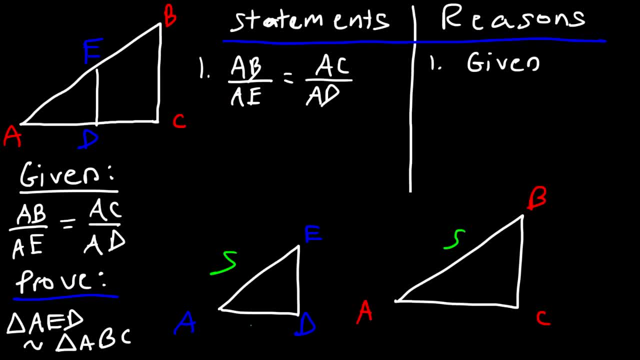 So then we can see that we might be able to use the side angle side postulate to prove that these two triangles are similar And notice that both triangles share a common angle And that's angle A. So in step two we could say that angle A is congruent to itself, based on the reflexive property. 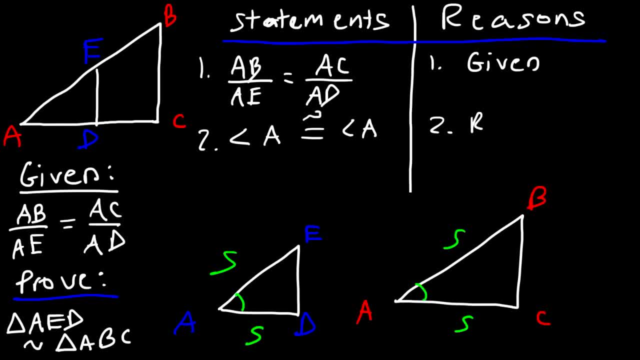 So in step two we could say that angle A is congruent to itself, based on the reflexive property. And so now we have enough to prove that the two triangles are similar using the side-angle-side. postulate The two sides. they have the same ratio, the two corresponding sides and the angles are congruent. 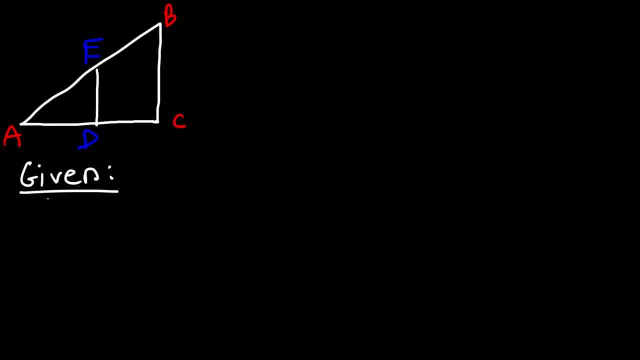 So for this problem, we're given the following information, And that is that AB divided by AE Is equal to AC divided by AD. So your task is to prove that triangle AED is similar to triangle ABC. So let's use a two-column proof. 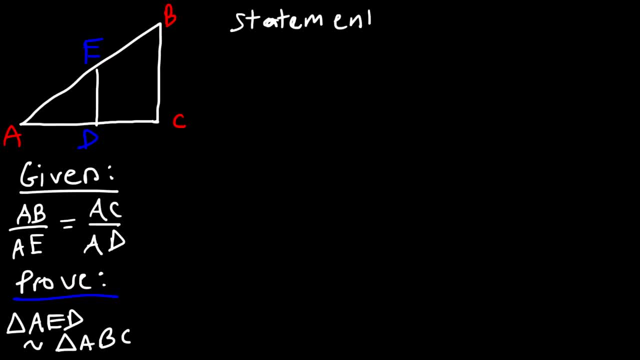 If you want to go ahead and try this problem. So let's start with the given, And that is: AB divided by AE is equal to AC over AD. Now let's draw the two triangles that we're trying to prove. So we're trying to prove that AED is similar to ABC. 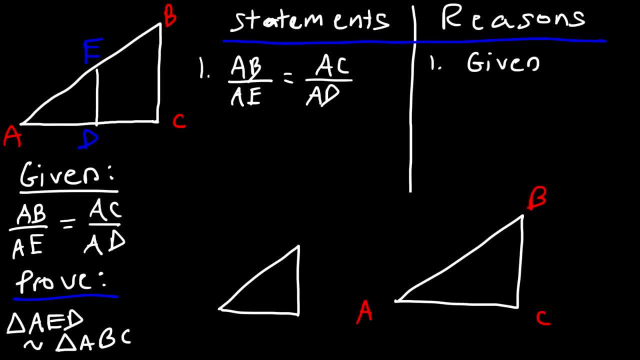 So this is ABC And this is AED And this is AED. Now, AB divided by AE is equal to AC divided by AD, So those two corresponding sides have the same ratio. based on this equation, So then we can see that we might be able to use the side angle side postulate to prove that these two triangles are similar. 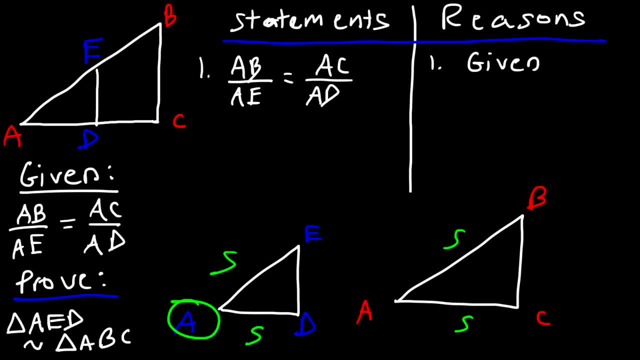 And notice that both triangles share a common angle, And that's angle A. So in step two we can say that angle A is congruent to itself, Based on the ratio Reflexive property. And so now we have enough to prove that the two triangles are similar. 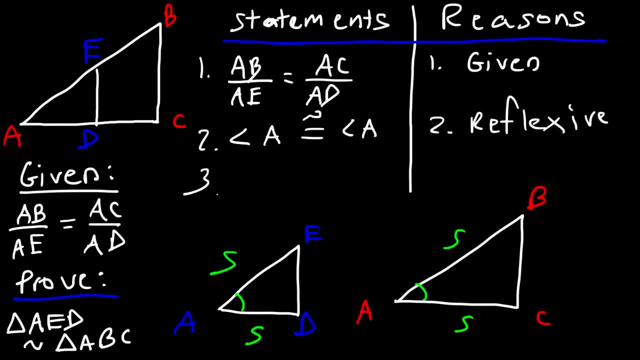 Using the side angle side postulate: The two sides. they have the same ratio, the two corresponding sides And the angles are congruent. So now we can say that triangle AED is similar to triangle ABC, And the reason for this it's the side angle side postulate. 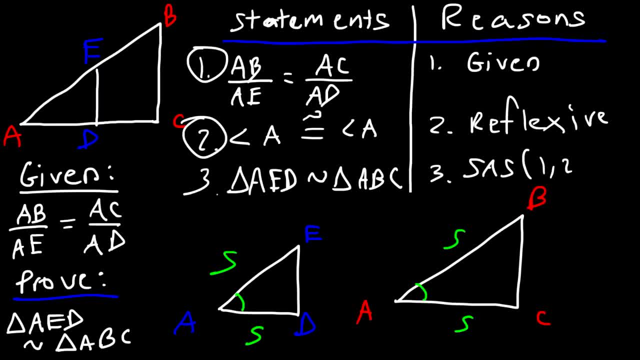 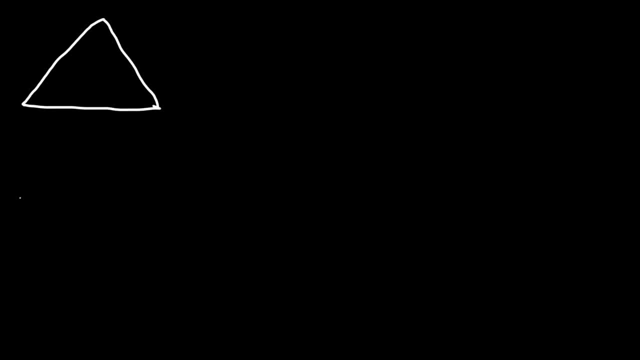 And the reason for this? it's the side angle side postulate, And we've used statements one and two to prove that. Now let's work on another two column proof that is not as long as the last one. So let's say this is triangle ABC. 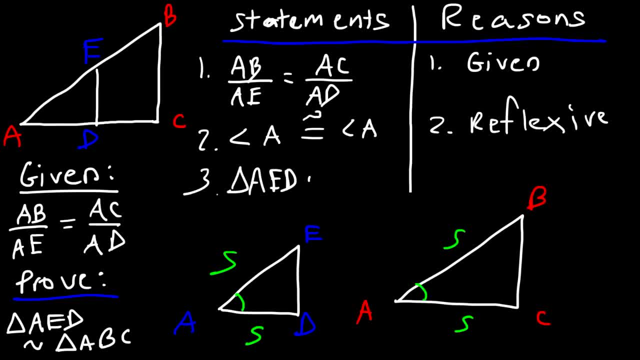 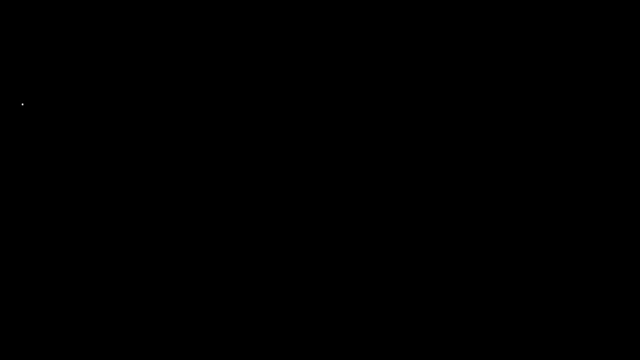 So now we can say that triangle AED is similar to triangle ABC, And the reason for this? it's the side-angle-side postulate, and we've used statements 1 and 2 to prove that. Now let's work on another two-column proof that is not as long as the last one. 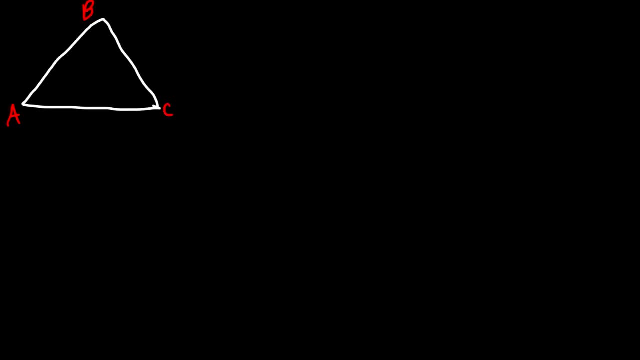 So let's say this is triangle ABC and we're going to have these two lines, Let's call this D and E, And so in this problem we're given the following information, And that is that AE and CD are altitudes. 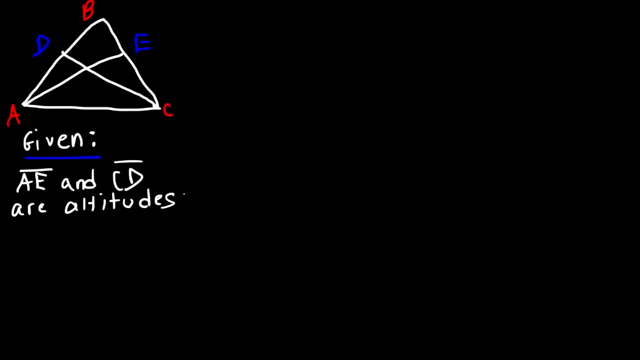 So, with this information, we need to prove that angle BAE is congruent to angle BCD. So how can we do so? Go ahead and try this problem. So let's start with the given information, And that is that AE and CD are altitudes. 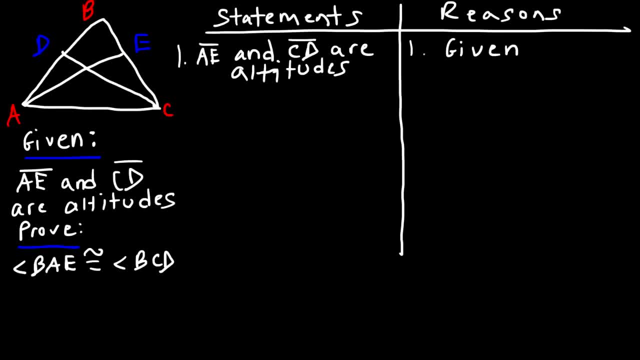 Now let's create a mental outline of the steps that we need to take in order to get the answer. So we need to prove that these two angles are congruent. So that's angle BAE and angle BCD. If we can prove that those two triangles are similar, then we can show that those two angles are congruent. 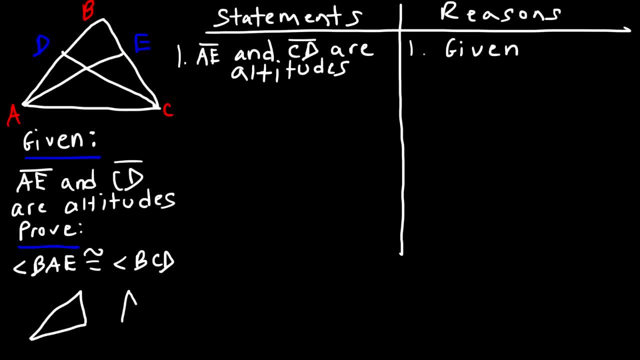 So let's draw those two triangles. So this is ABE and here we have CBD. So now, what do we know about altitudes? Altitudes form right angles with the side that's opposite to the vertex. So A is a vertex and the side opposite to it is BC. 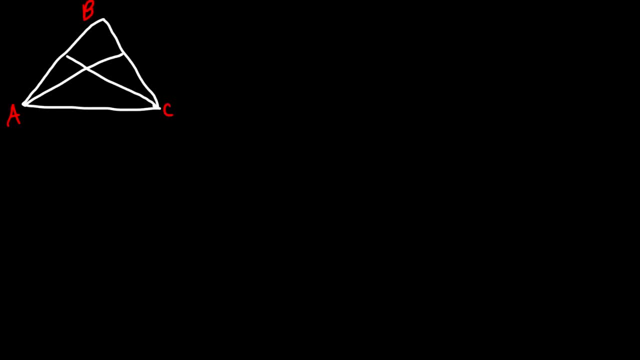 And we're going to have these two lines, Let's call this D and E. And so in this problem we're given the following information, And that is that AE and CD are altitudes. So with this information we need to prove that angle BAE is congruent. 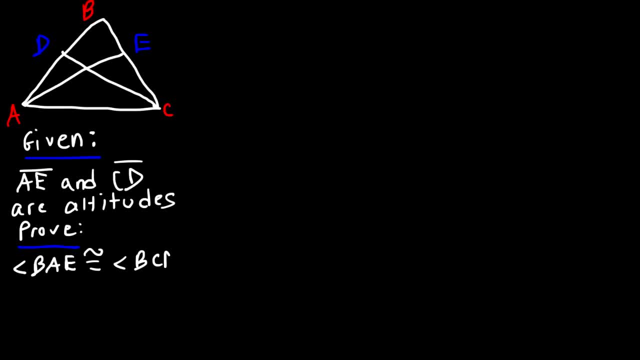 And that angle BAE is congruent To angle BCD. So how can we do so? Go ahead and try this problem. So let's start with the given information, And that is that AE and CD are altitudes. Now let's create a mental outline of the steps that we need to take in order to get. 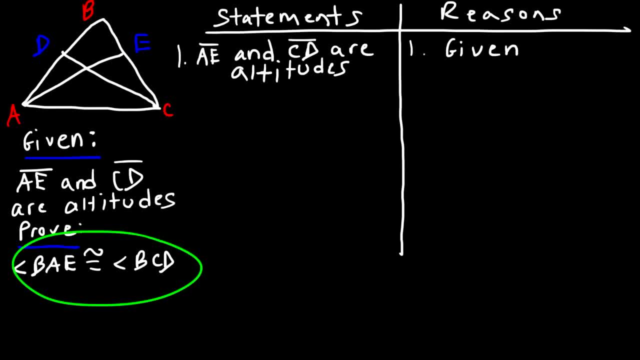 the answer. So we need to prove that these two angles are congruent. So that's angle BAE and angle BCD. If we can prove that those two triangles are similar, then we can show that those two angles are congruent. 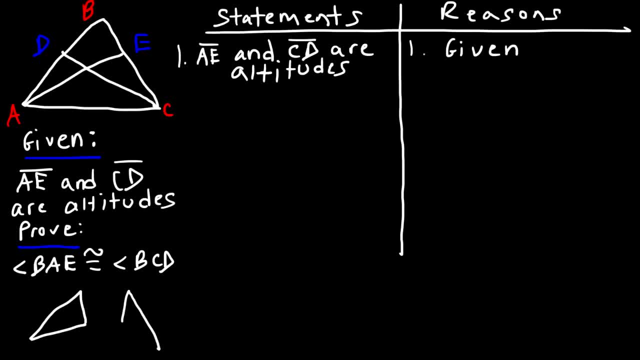 So let's draw those two triangles. So this is ABE, and here we have CBD. So now, what do we know about altitudes? Altitudes form right angles with the side that's opposite to the vertex, So A is a vertex. 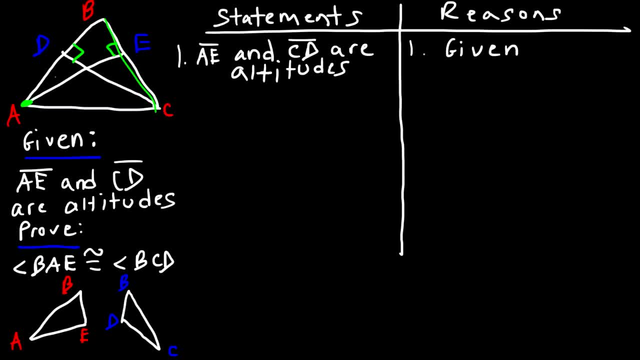 And the side opposite is a vertex. So A is a vertex And the side opposite to it is BC. So altitude AE is going to be perpendicular to BC, And the same is true for the other altitude. So therefore we could say that angle BDC, which is this angle, and angle BEA, which 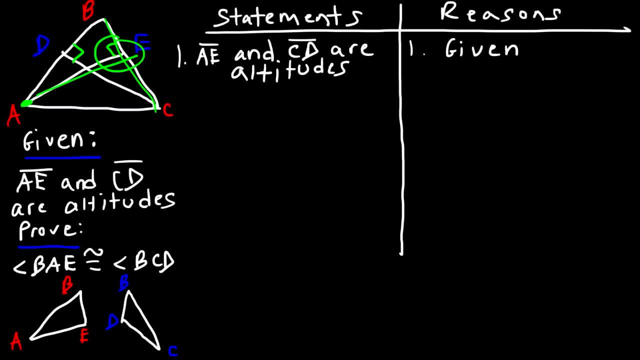 So altitude AE is going to be perpendicular to BC, And the same is true for the other altitude. So therefore we could say that angle BDC, which is this angle, and angle BEA, which is this angle, those two angles are right angles. 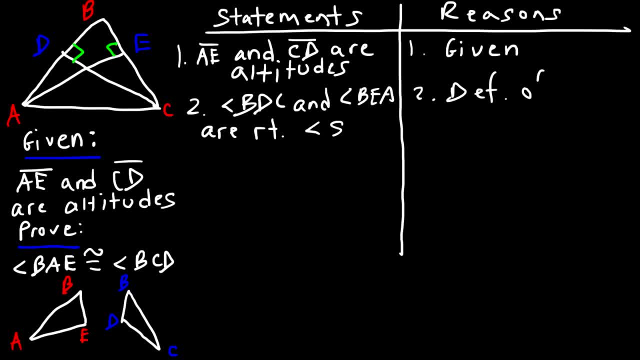 And the reason for this Definition Of an altitude: Altitudes. they form right angles with the side opposite to the vertex. Now, because those two angles are right angles, they have to be congruent to each other. So we could say that angle BDC is congruent to angle BAE. 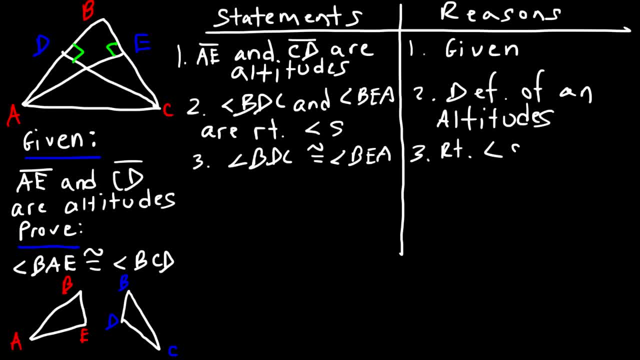 And the reason: Right angles are congruent, So let's mark that. So this is BDC And this is BEA, So those two are congruent. Now, these two angles are common to both triangles. So in step four we could say that angle B is congruent to itself, based on the reflexive property. 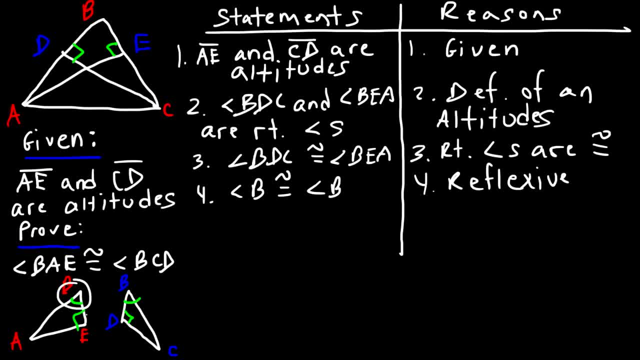 So now we've shown that two angles of these two triangles are congruent, So we can now make the statement that those two triangles are similar. So in step five we are going to say that triangle BDC is similar to triangle BEA. 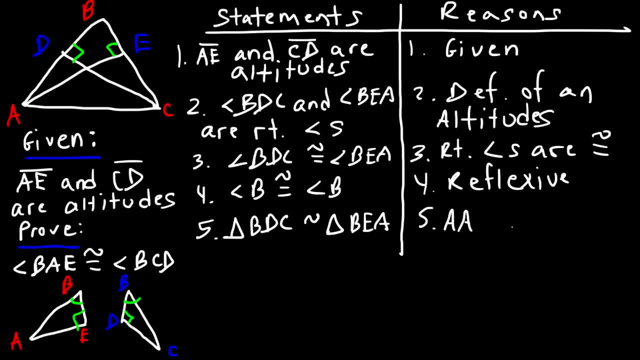 And this is based on the angle-angle postulate for triangle similarity, and we've used Statements 3 and 4 to establish it shape. So now that we've shown that the two triangles are similar, we can now state that any of its angles are congruent. So therefore, these two angles must be congruent, So we can. 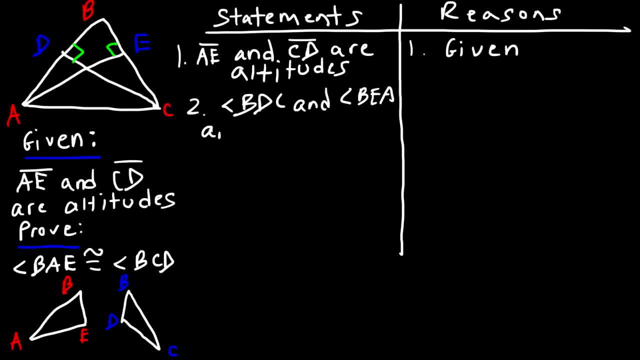 is this angle, Those two angles. Those two angles are right angles And the reason for this definition of an altitude- Altitudes- they form right angles with the side opposite to the vertex. Now, because those two angles are right angles, they have to be congruent to each other. 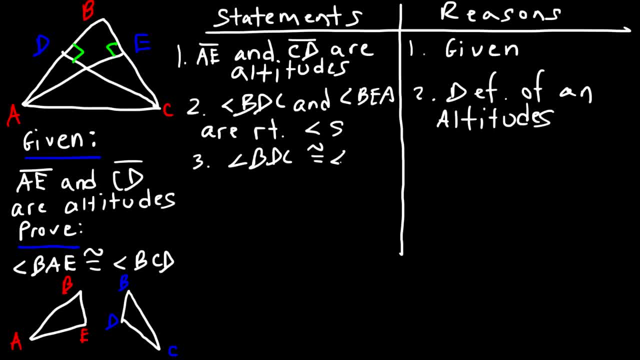 So we could say that angle BDC is congruent to angle BAE, And the reason: Because those two angles are congruent. So let's mark that. So this is BDC and this is BEA, So those two are congruent. 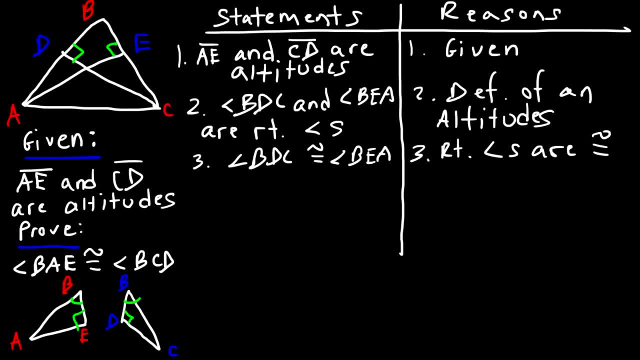 Now these two angles are common to both triangles. So in step four we could say that angle B is congruent to itself Based on Based on the reflexive property. So now we've shown that two angles of these two triangles are congruent. 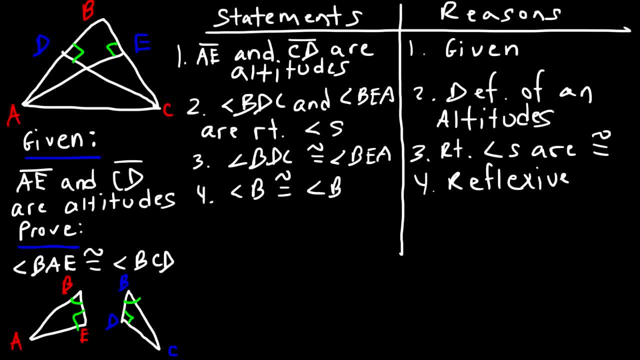 So we can now make the statement that those two triangles are similar. So in step five we're going to say that triangle BDC is similar to triangle BEA. This is based on the angle-angle postulate for triangle similarity And we've used statements three and four to establish it. 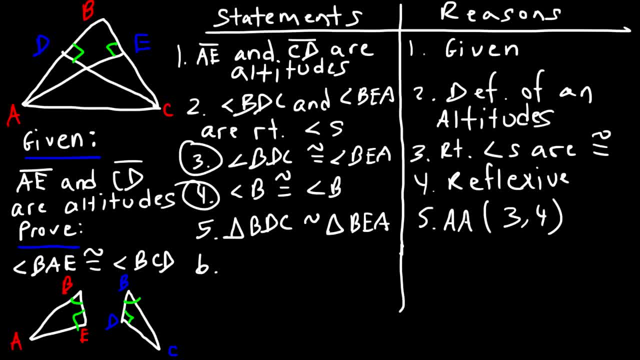 So, now that we've shown that the two triangles are similar, we can now state that any of its angles are congruent. So, therefore, these two angles must be congruent, So we can now make the statement that angle BAE, which is this one, is congruent to this. 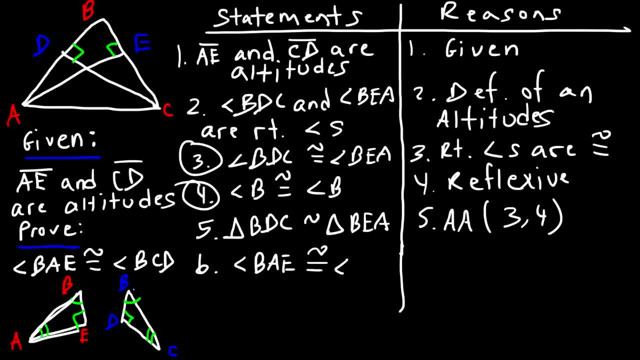 angle Is congruent to angle BCD, And what reason can we write in the second column? Well, we could say this: Correspondence sides of similar triangles are congruent. So after you prove that two triangles are similar, You can state that 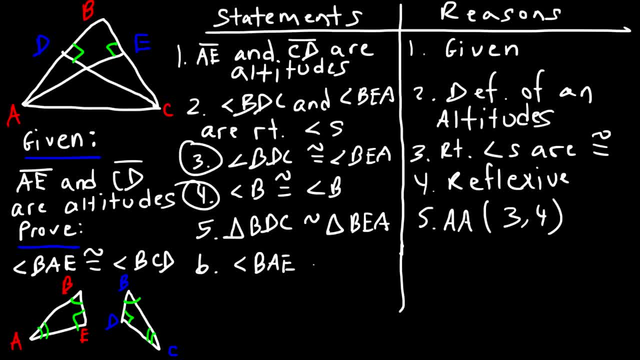 now make the statement that angle BAE, which is this one, is congruent to angle BCD. And what reason can we write in the second column? Well, we could say this: Correspondent sides of similar triangles are congruent. So after you prove that two triangles are similar, 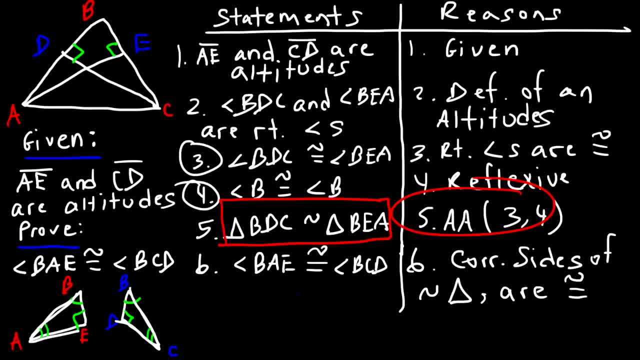 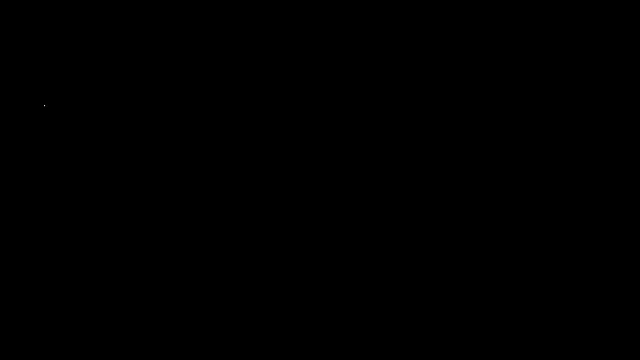 you can state that any of its corresponding angles are congruent, And so that's it for this problem. Let's work out one more proof. So, as usual, let's say this is A, B and C, And let's draw a horizontal line in the middle. 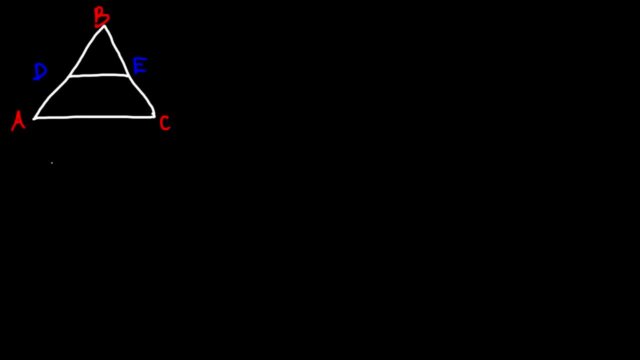 And so this is going to be D and E. So in this problem we are given that D? E is parallel to A C And we need to prove that the product of A, B and B E is equal to the product of B C and B D. 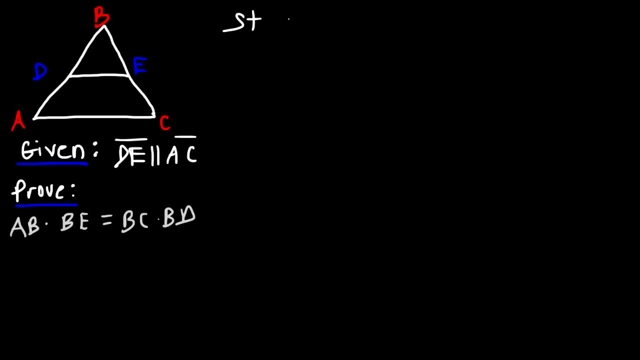 So what do you think we need to do in order to show that the product of A, B and B E is equal to the product of B C and B D, And in order to show that the last statement is true? 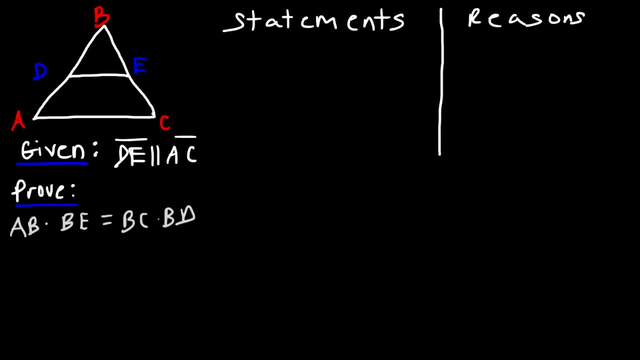 Well, let's find out. So let's start with our given, And that is that D: E is parallel to A C, And so let's put some marks on the figure. So let's start with our given, And that is that D: E is parallel to A C. 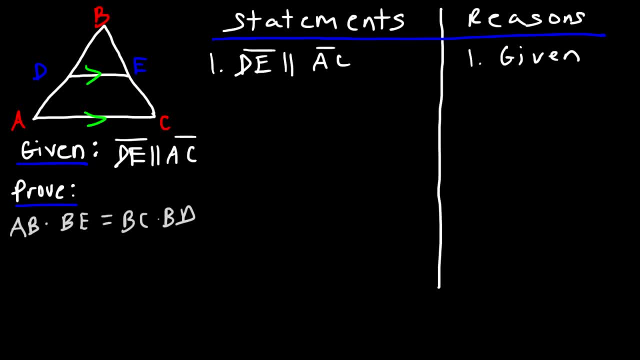 And so let's put some marks on the figure Now, because the two lines are parallel. that means that there's going to be some angles that are congruent, And so it turns out that these two angles are congruent to each other. They're corresponding angles. 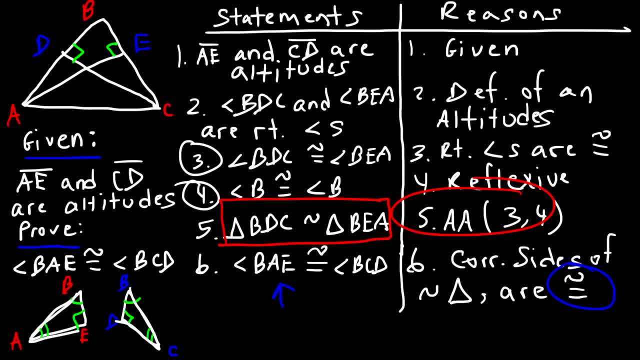 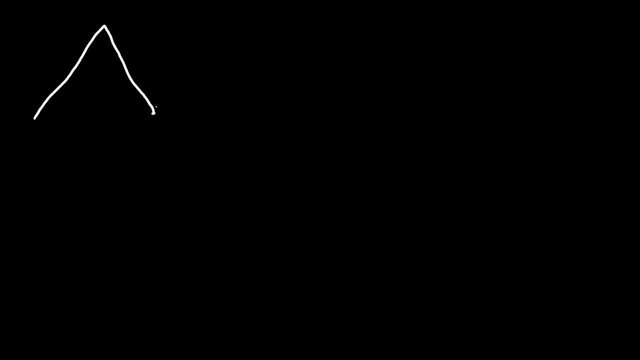 Any of its corresponding angles are congruent, And so that's it for this problem. Let's work out one more proof. So, as usual, let's say this is A, B and C, And let's draw a horizontal line in the middle. 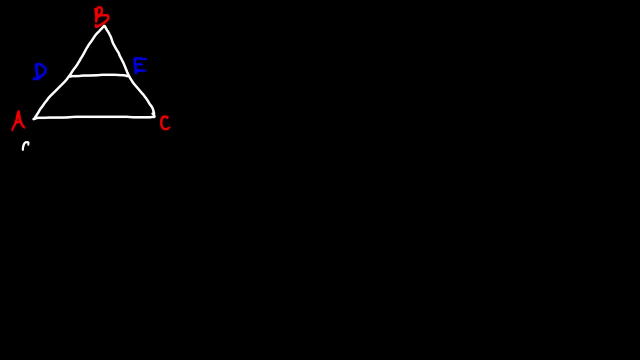 And so this is going to be D and E. So in this problem, We are given that DE is parallel to AC And we need to prove that the product of AB and BE is equal to the product of BC and BD. So what do you think we need to do in order to show that the last statement is true? 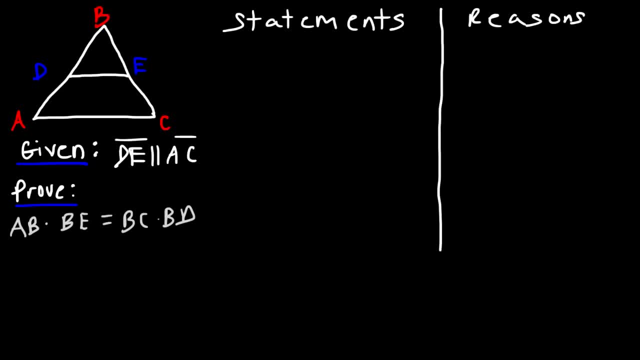 Well, let's find out. So let's start with our given, and that is that DE is parallel to AC, And so let's put this into historic form. Let's start with our learned error of D. Well, if we work this out, let's see. 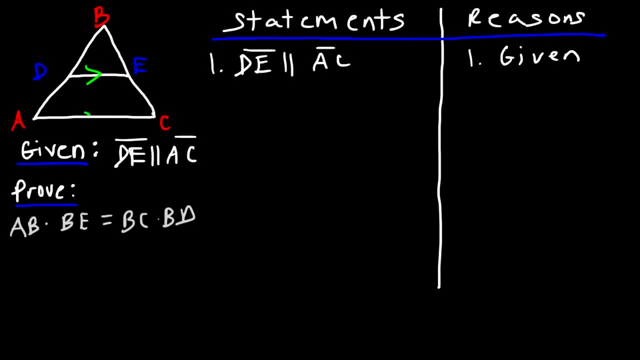 We took the greater part of the basicugo. Let's say we took R10.. Let's put some marks on the figure Now. because the two lines are parallel, that means that there's going to be some angles that are congruent, And so it turns out that these two angles are congruent to each other. 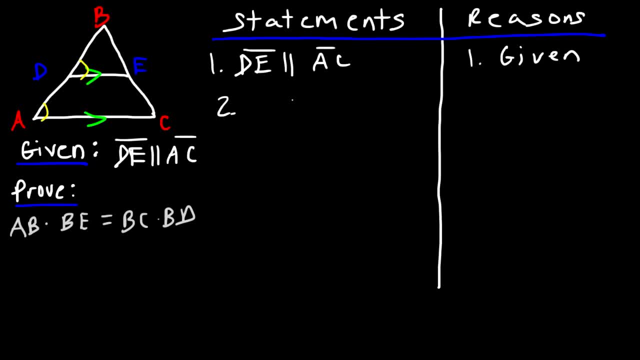 They're correspondent angles. So in step two we could say that angle BDE, which is this angle that's congruent to angle A, And the reason is: since we have parallel lines, the corresponding angles are congruent. Now let's move on to step three. 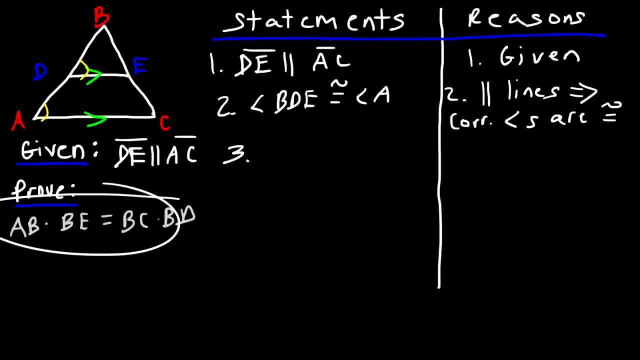 Now let's draw a picture In order to prove this statement. we need to prove that two triangles are similar, So we need to prove that the small triangle is similar To the large triangle. So the small triangle is going to be triangle DBE, which is this triangle here. 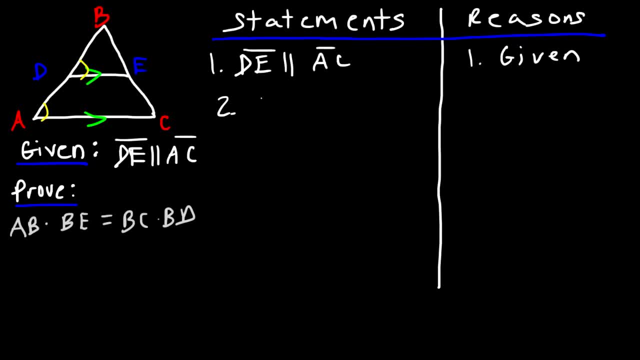 So in step two we could say that angle BDE, which is this angle that's congruent to angle A, And the reason is: since we have parallel lines, the corresponding angles are congruent. Now let's move on to step three. 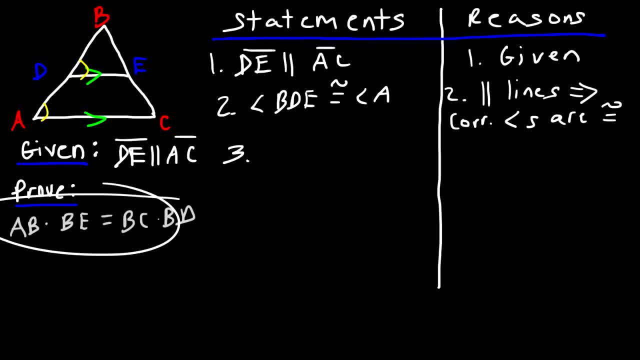 Now let's draw a picture In order to prove this statement. we need to prove that two triangles are similar, So we need to prove that the small triangle is similar to the large triangle. Okay, So the small triangle is going to be triangle DBE, which is this triangle here. 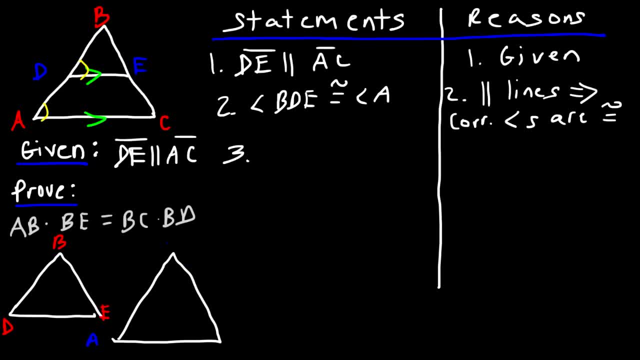 And we need to show that it's similar to the large triangle ABC. So right now we've shown that angle BDE is congruent to angle A. Now notice that these two triangles share a common side and that is angle B. So in step three we could say that angle B is congruent to itself, based on the reflexive 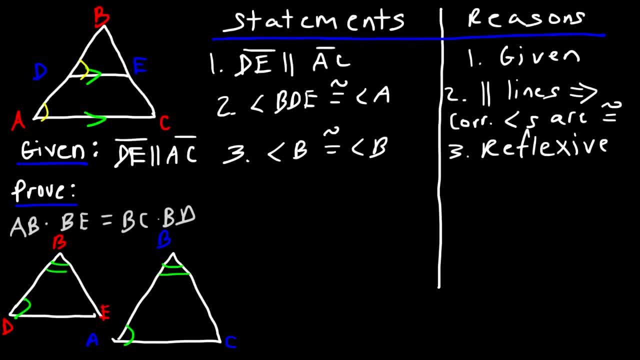 property. So now that we know that the two angles of these two triangles are congruent, we can make the statement that the two triangles are similar. So in step four, let's say that triangle BDE is similar to BDE. So this is based on the angle-angle postulate, using statements two and three. 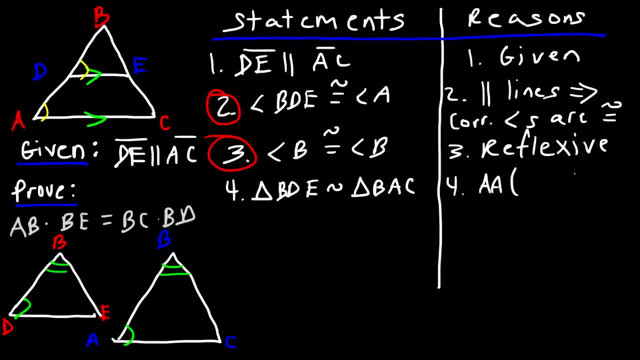 So now let's move on to step five. So what do we need to do at this point? Because the two triangles are similar, we could say that they're congruent. Okay, We could say that their corresponding sides are proportional. So we could say that AB to BD, they have the same ratio as BC and BE. 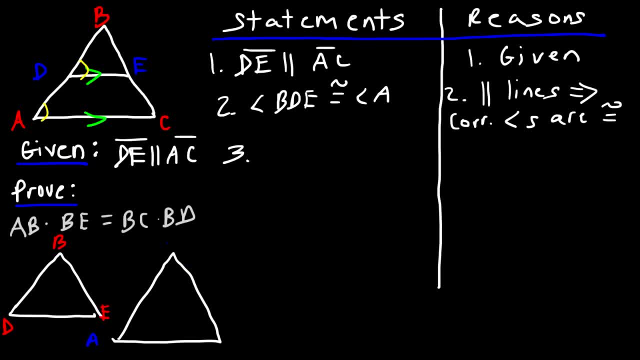 And we need to show that it's similar to the large triangle ABC. So right now we've shown that angle BDE is congruent to angle A. Now notice that these two triangles share a common side And that is angle B. So in step three we could say that angle B is congruent to itself, based on the reflexive 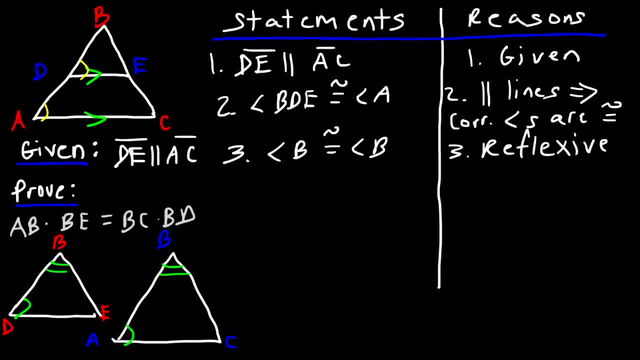 property. So now that we know that the two angles of these two triangles are congruent, we can make the statement that the two triangles are similar. So in step four, let's say that triangle BDE- BDE- is similar to triangle BAC, and so this is based on the angle angle postulate. 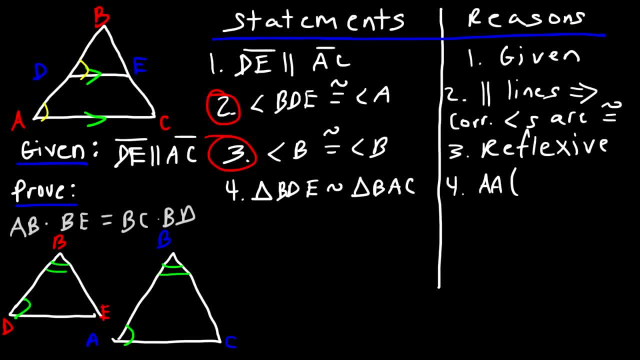 using statements 2 & 3. so now let's move on to step 5. so what do we need to do at this point? because the two triangles are similar, we could say that the corresponding sides are proportional. so we could say that, a being to be, D, they. 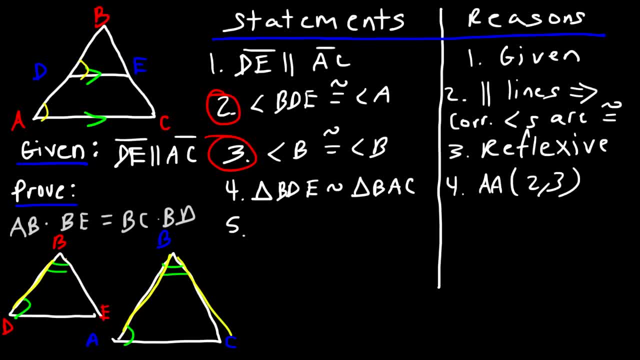 have the same ratio as BC and be. so a be divided by DB or BD, that's for these two sides. the ratio between those two is going to be the same as the ratio between BC and be. so a be over BD is equal to BC over be. and for step 5 we 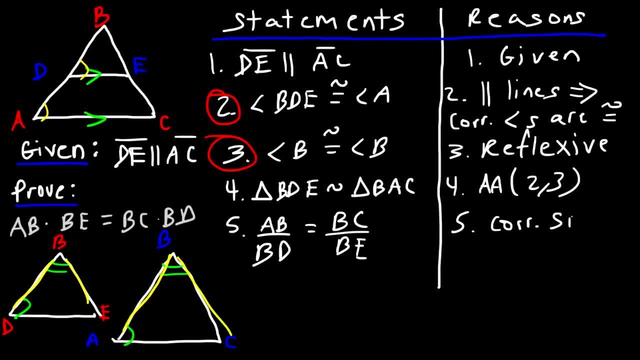 could say that the corresponding sides of similar triangles are proportional. so now we can move on to step 6 and let's cross. multiply these two fractions, so a, b x BED is equal to BC times ED, and this is known as the meeting between better and worse, and B1 and B2 is the most special fraction here. so AB times BE is equal to BC times BD, and this is known as the major fraction. so AB times DE is equal to 174 times or 20 times hp is respect to 107 times%. yay. 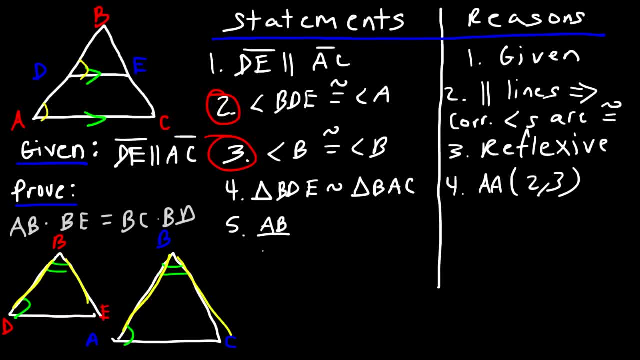 So AB divided by DB or BD. so that's for these two sides. the ratio between those two is going to be the same as the ratio between these two. Okay, The ratio between BC and BE. So AB over BD is equal to BC over BE. 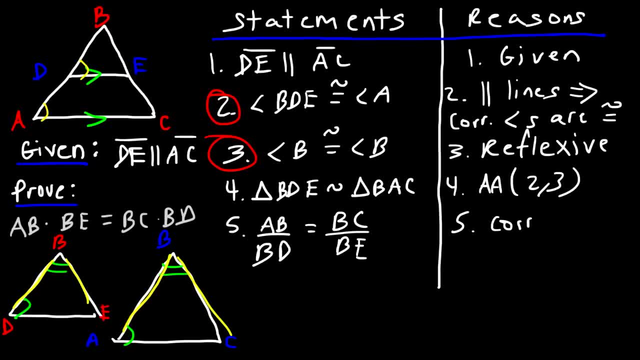 And for step five we could say that the corresponding sides of similar triangles are proportional. So now we can move on to step six, And let's cross-multiply these two fractions, So AB times BE is equal to BC times BD, And this is known as the means-extremes product theorem. 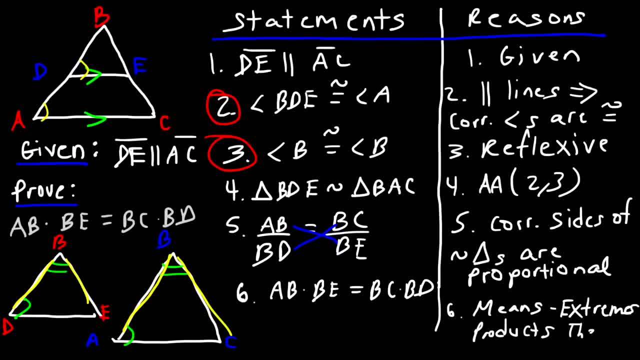 Okay, So that's how you can prove this statement. So once you show that the two triangles are similar, you could show that the corresponding sides are proportional And, rearranging this equation based on the means-extremes product theorem, you could show that this relation is true. 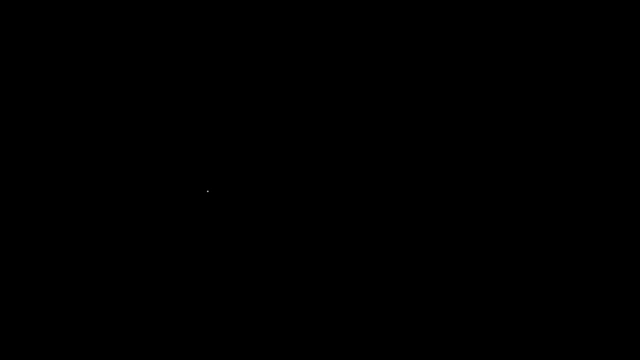 And so that's how you can prove that statement. So let's say: if you have A over B, which is equal to C over B, So let's say if you have A over B, which is equal to C over B, Okay, 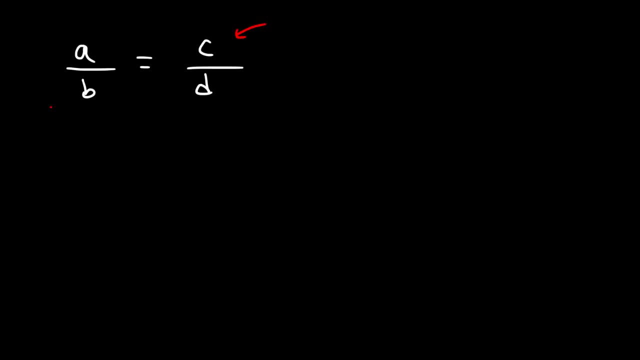 So let's say, if you have A over B, which is equal to C over D, These two are known as the means And these two are known as the extremes. So you can rewrite this equation like this. You could say: E1, that's one of the extremes, over M1 is equal to M2, the other mean over. 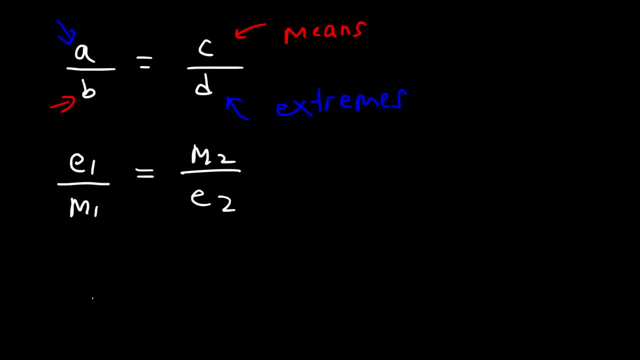 the other extreme, E2.. Now if you cross-multiply, you're going to get M1 times M2. So that's the product of the means. And then if you multiply these two, you're going to get the product of the extremes. 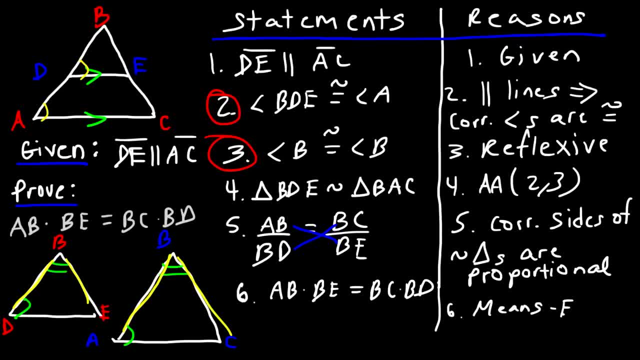 the means extremes product theorem. so that's how you can prove this statement. so once you show that the two triangles are similar, you could show that the corresponding sides are proportional and, rearranging this equation based on the means extremes products theorem, you can show that this relation is true. and so 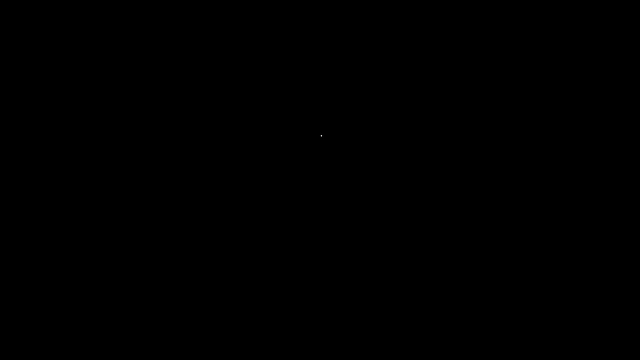 that's how you can prove that statement. so let's say: if you have a over B, which is equal to C over D, these two are known as the means and these two are known as the extremes. so you can rewrite this equation like this. you could say: e1. 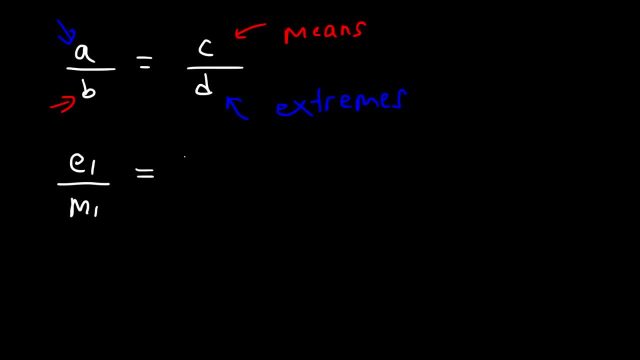 that's one of the streams over. m1 is equal to m2. the other mean over the other extreme, e2. now if you cross, multiply you're going to get m1 times m2, so that's the product of the means. and then if you multiply these two you're going to get the products of the. 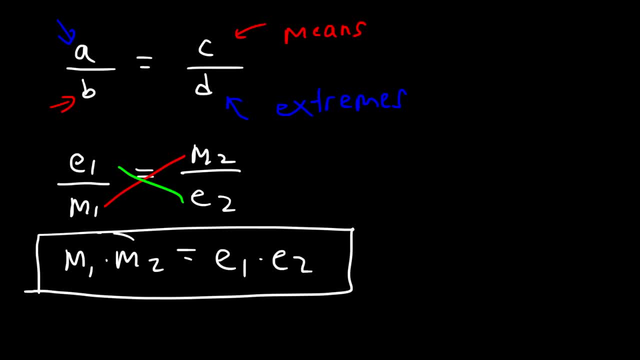 extremes. so the products of the means m1 times m2 is equal to the product of the extremes e1 times e3, and so you can see the relationship between, or why it's called the means extremes products theorem. and so that's all I got for this video. hopefully you 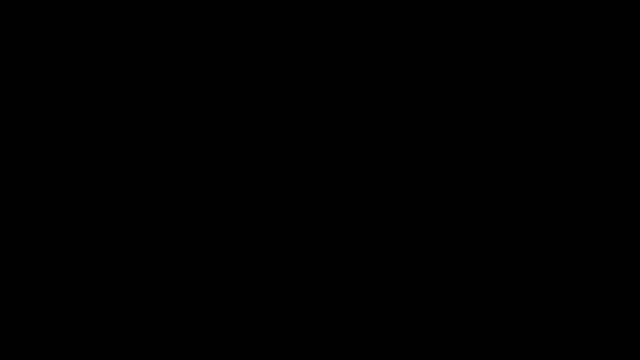 found it to be useful. thanks for watching and I'll see you in the next video. 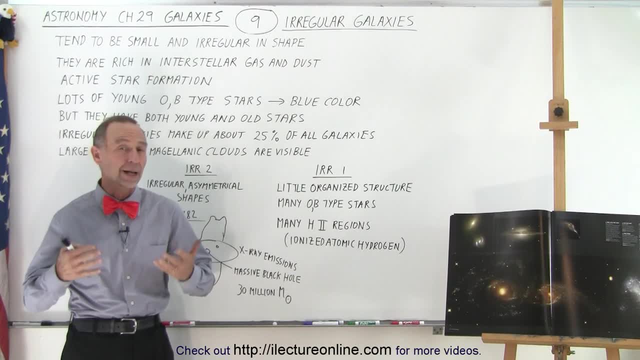 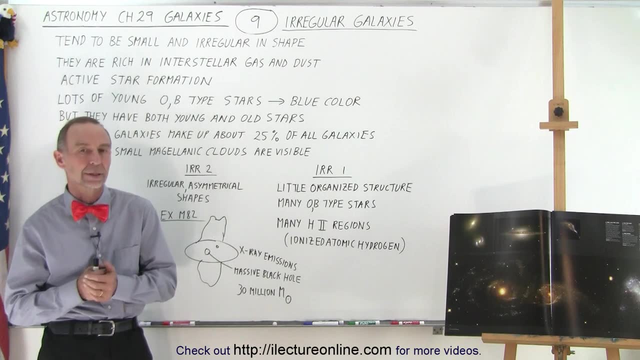 Welcome to our lecture online. Now let's take a look at the third type of galaxy. We saw the elliptical galaxy. we saw the spiral galaxies. now we're taking a look at the irregular galaxies And of course, the name indicates that they don't have a specific shape. they're irregular in shape.